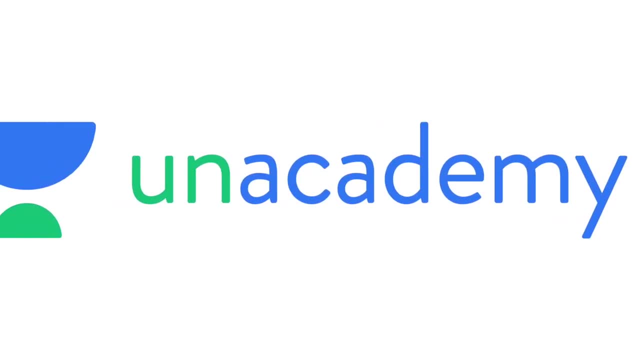 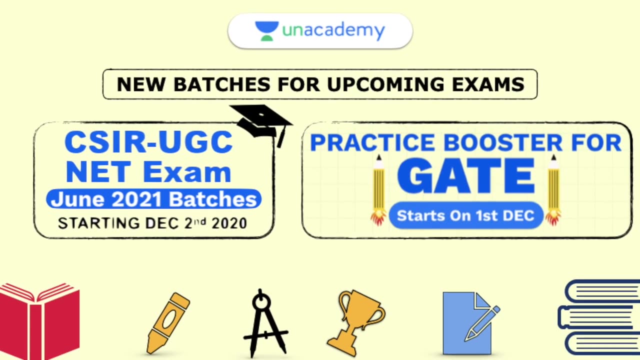 telling you anything about the this particular topic. let me tell you about my classes which are running right now on an academy plus. so i have started two new batches for gate and for cs iron, at both exam preparation. so if you are interested in joining those classes you can take an academy plus subscription using my 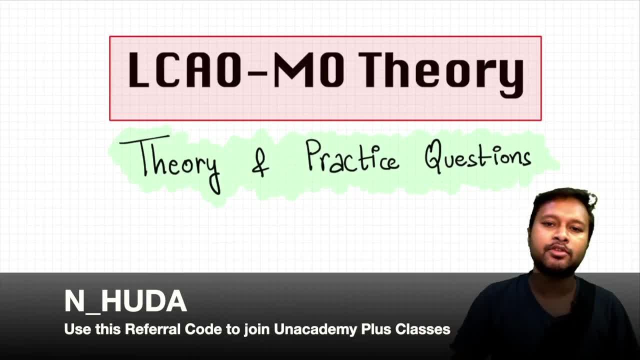 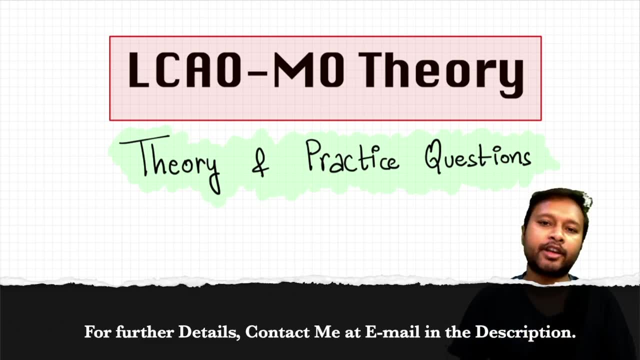 referral code that is n underscore huda, so you can use that particular referral code to take an academy plus subscription and you can access my classes on an academy. for more details you can contact me on the email id provided in the description of this video. all right, so having 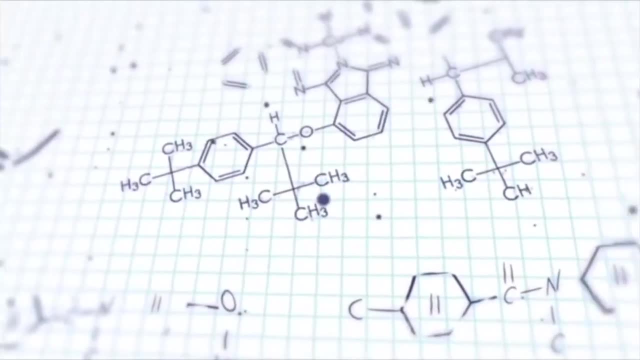 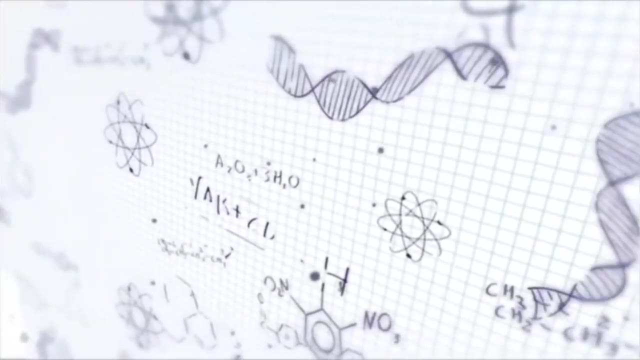 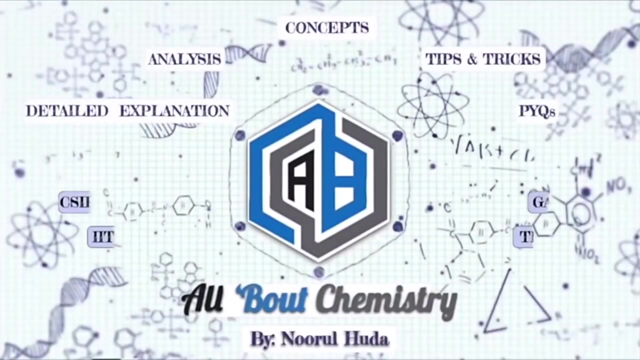 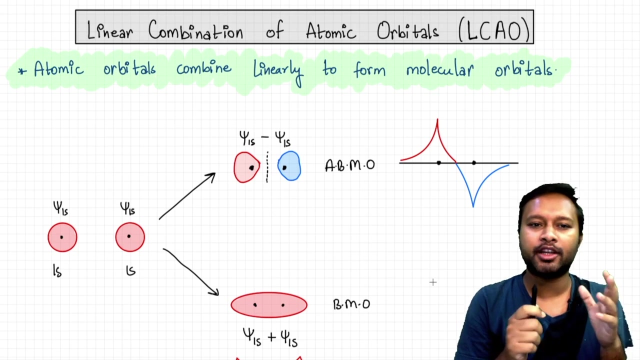 said that let's continue with our video. all right, so we will start from this particular interactive slide over here, uh, which talks about the linear combination of atomic orbital. so if you understand, if you have read about molecular orbital theory anywhere in your chemistry or in your chemical bonding or in your quantum mechanics, like in any of the aspect, 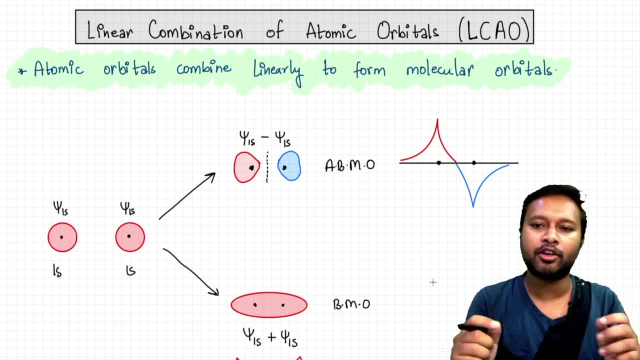 so the basic explanation or the basic definition of the molecular orbital theory says that you will be having atomic orbitals which are going to linearly combine- okay, and they are going to form molecular orbitals. now these linear combination of atomic orbitals can be done in two ways: can be done constructively or it can be done destructively. 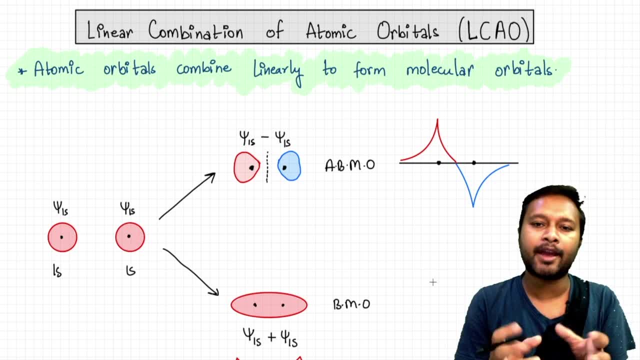 so, based upon constructive and destructive, like overlapping, you will have two different types of molecular orbitals. you will have bonding molecular orbital and you will have anti-bonding molecular orbital. now, that's what the basic theory is all about. okay, so atomic orbitals getting combined linearly. what does that? linearly means? means head to head. they are going. 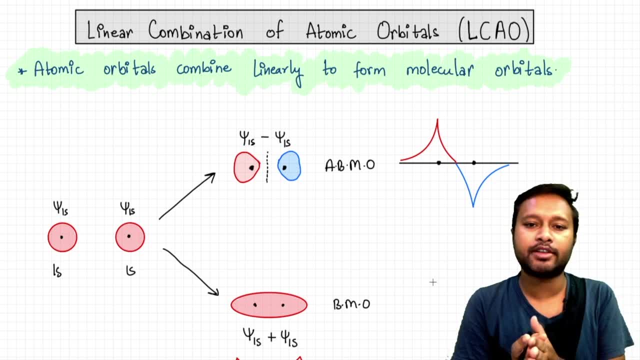 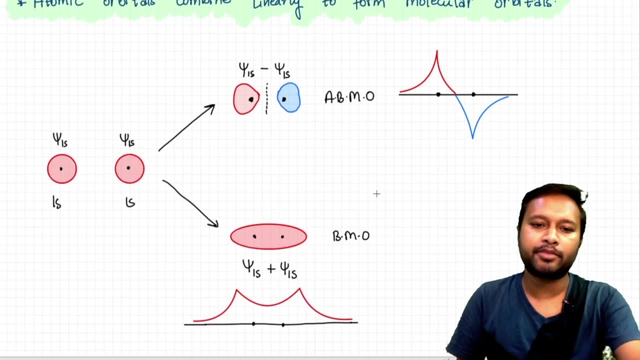 to combine. okay, and this linear combination of these atomic orbital give rise to the molecular orbitals, and molecular orbitals can be bonding or anti-bonding. now, if you look upon this particular diagram, so here i have made 1s orbitals. now, these two 1s orbitals, which 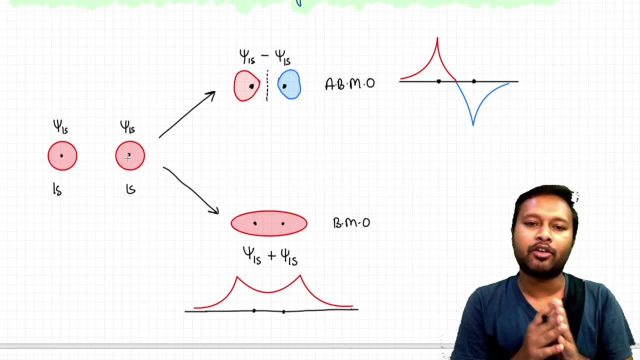 you can see over here, which are shown by the red spheres. now red color of orbitals. wherever i will show you in this particular whole video, red color will signifies you positive, lobe, or the positive like side of the orbital, and blue color is going to show you the negative side. okay, so blue color. 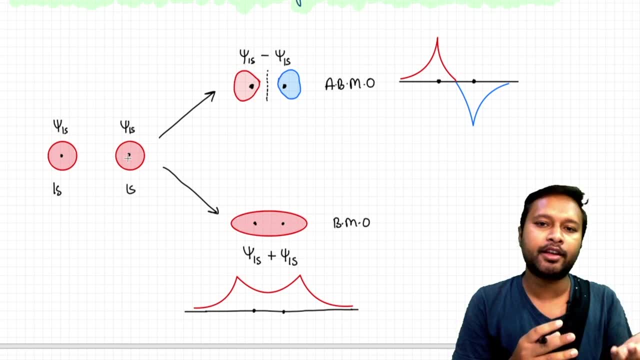 is going to show you the negative lobes, and red color is going to show you the positive lobes, and blue color is going to show you the negative lobes, and red color is going to show you the negative lobes, wherever it will be now, if you see here. so these, both these s orbitals are there. 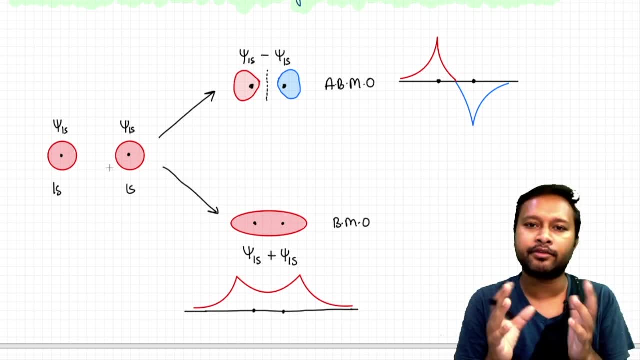 s orbitals are positively like. it has a positive electron cloud around it. now then, the blue color is also there, but that is deeply buried inside, so that's why we cannot see that. so overall, it looks like a spherical red color, right like the, the positive charge like surrounding this s orbital. 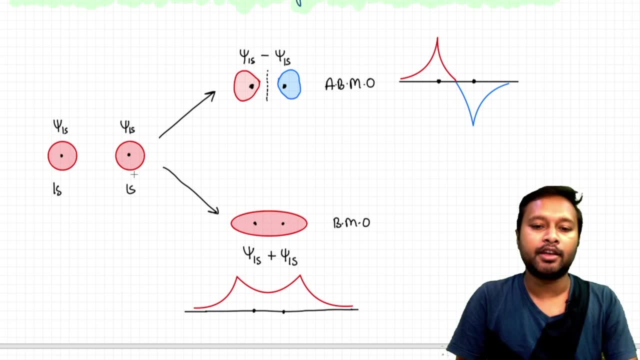 now these two s orbitals. when they linearly combine, they are going to form a pair of like bonding molecular orbital and a anti-bonding molecular orbital. now this bonding molecular orbital is done when there is a addition of these two wave functions. now let's talk about 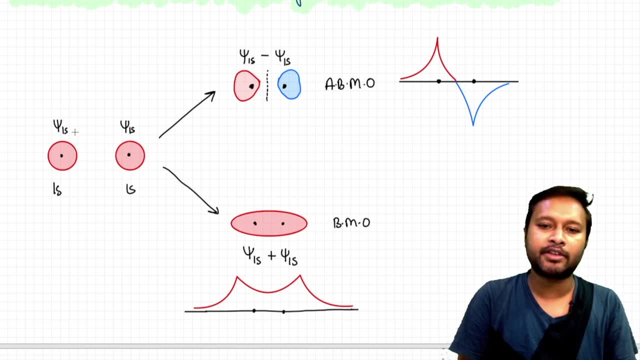 it from the like quantum mechanical point of view. so let's say i have expressed it as wave function, psi 1s and this is also psi 1s. okay, so for just to make sure that you can differentiate between both of them, let me put a dash over here. so this is psi 1s and this is psi 1s. dash. now, these are the two. 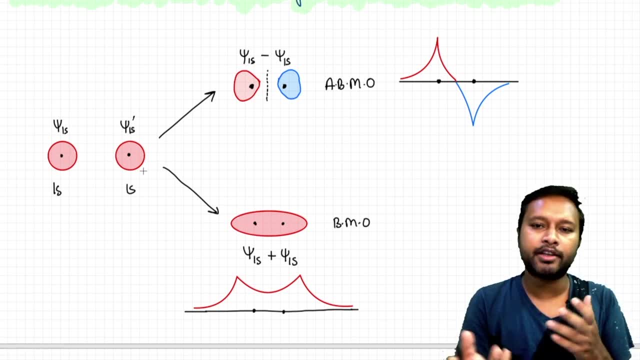 wave function of two, like having 1s, 1s orbital. Now when they are going to combine they can combine as psi 1s plus psi 1s, psi dash 1s. So that means both of them have combined constructively over here. Now when they 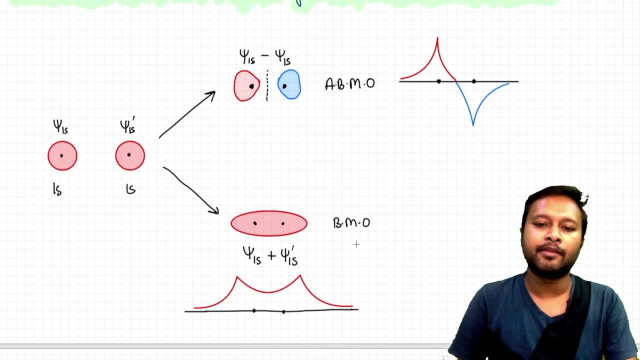 form constructive overlapping or constructive combination. they are going to give a bonding molecular orbital because its energy will be lower. Now the other one which we will be having will be psi 1s minus psi dash 1s. Now, in this case, they are going to form anti-bonding molecular 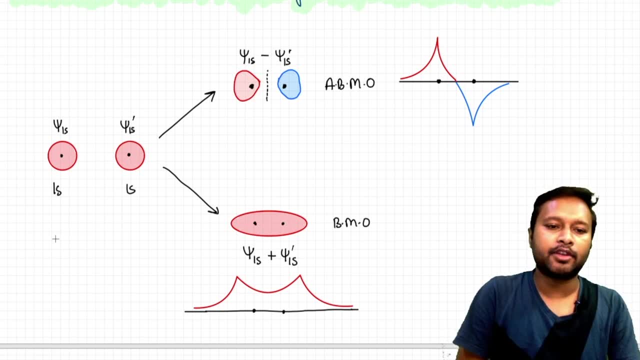 orbital. Now how does the wave function is going to look like? So if the wave function like representing your 1s orbital is like this and the wave function representing the this particular 1s orbital is like this, So their constructive overlapping is going to form a wave function. 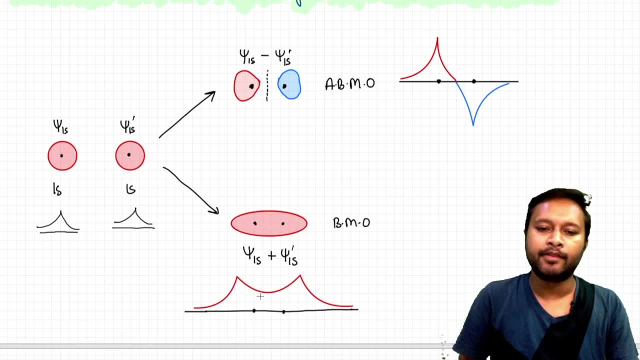 which is shown with this particular red colored wave. So this is how the bonding molecular orbital wave function is going to look like, and for anti-bonding molecular orbital, you can see that the wave function is going to be something like this, having a positive side and a negative. 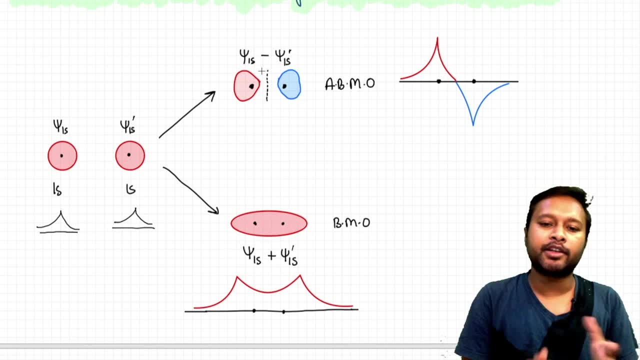 side. Now, if you look upon the, the visual diagram of it, it shows something like this: in the constructive overlapping you have this whole surface like having similar charge. So the electron cloud is basically surrounded by the whole, like it's surrounded in the oval shape, and these two dots are just like the foci of the. 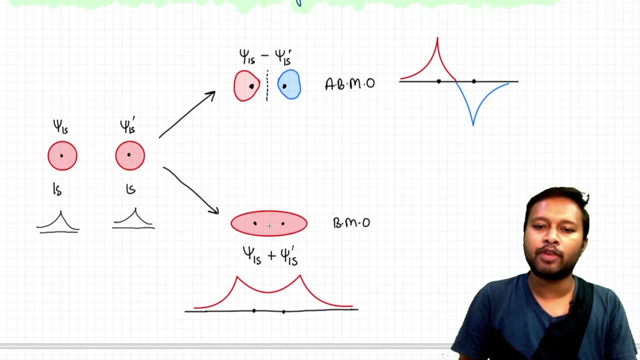 ellipse. So these two dots are basically showing you the two atoms. Now here, these two dots are obviously at their own positions, but here the orbitals have destructively overlapped. So that's why this particular one is 1s and this is 1s dash in the destructive manner. 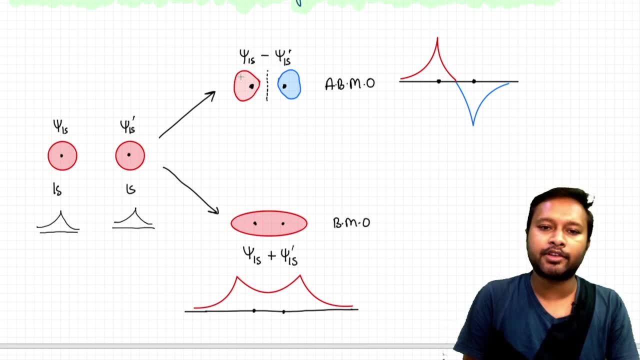 that is minus 1s dash, and in the center of that. so this is positively charged, this is negatively charged. in the center of them there will be a place, or there will be a plane where there is no probability of finding electron, So that particular plane is called as your nodal surface. 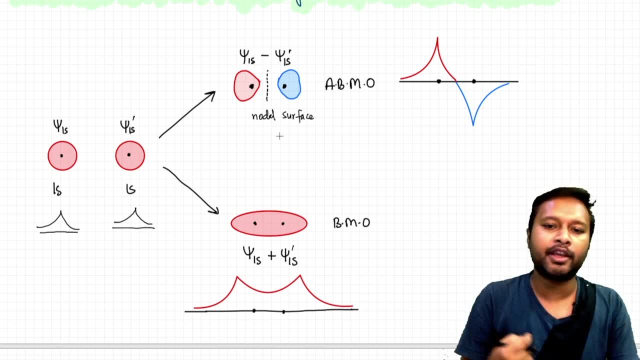 okay, that is going to be nodal surface or nodal plane or nodal point, okay. So there are many definitions of it, depending upon what you are talking about: whether you are talking about a line, whether you are talking about a plane or a surface. So this nodal can be decided like that. 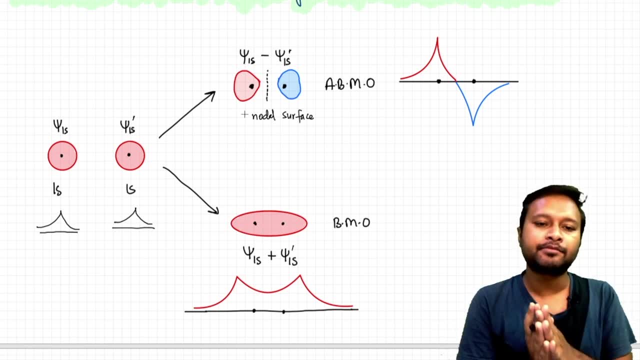 So remember one thing. I just want to give you some definitions over here. First of all, what is orbital? okay, what is an orbital according to quantum mechanics? So orbital is a radial extent around an atom up till which probability of finding electron is there. okay, So that's what. 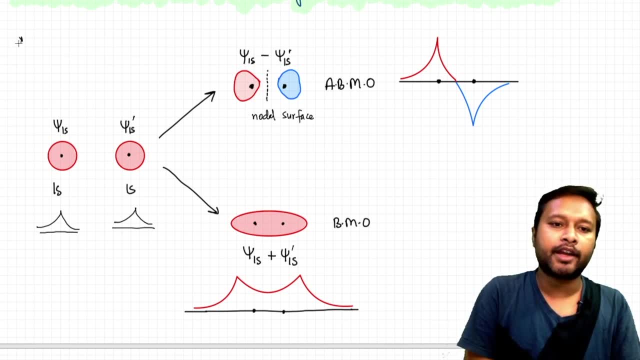 an orbital is. So let me just write it down here that the space, okay, the space around an atom is an atom where probability of finding an electron is okay, where probability of finding an electron is like is present, okay, or basically there is some probability of finding an electron. 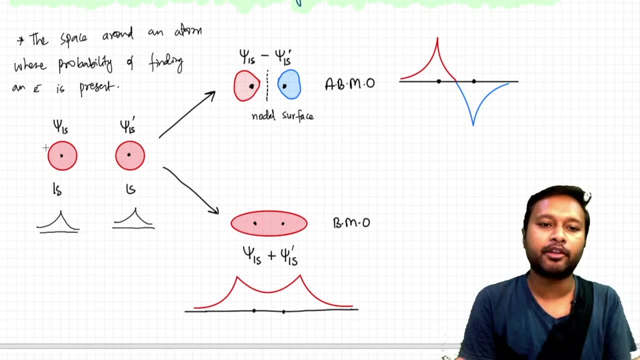 in that particular space, that particular space or that particular radial extent. This is space. you can also write down as radial extent. okay, So this particular thing is called your orbital. So orbital is nothing, but it is telling you that up till where or up till what. 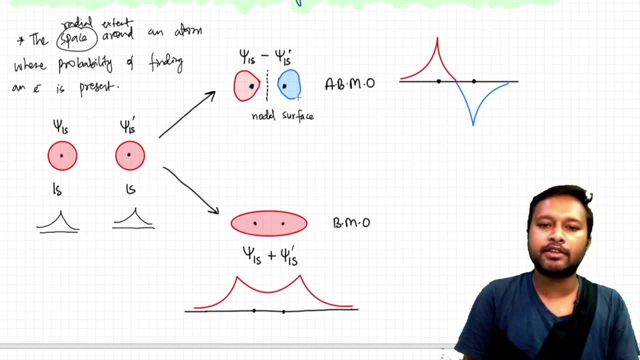 surface, there is a probability of finding electron. So these shaded regions are basically showing you that up till which region or up till what extent you can find an electron. that is what it is all about. Now, once we have understood this particular thing, now you can understand for the p orbital. 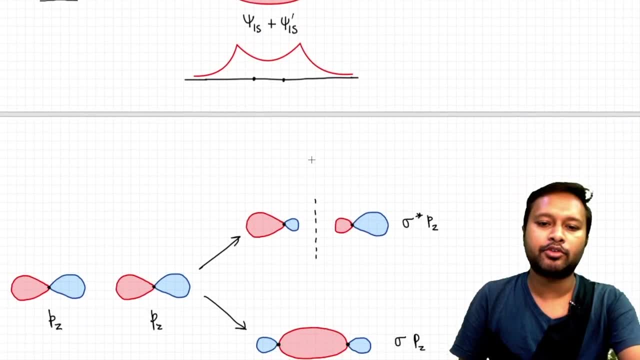 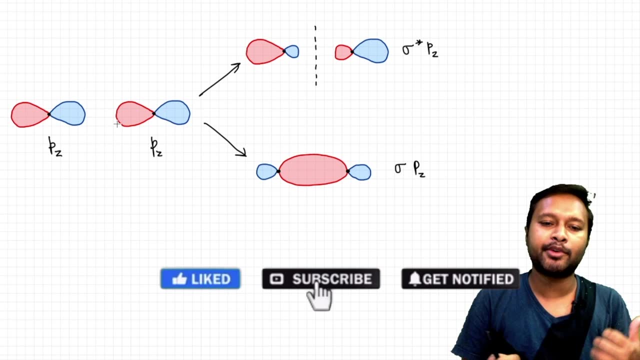 like forming bonding and anti-bonding orbitals. So let me show you that as well. So let us say the p? z orbitals. So p z orbitals are going to form the sigma bonding. Why? Because they do head. 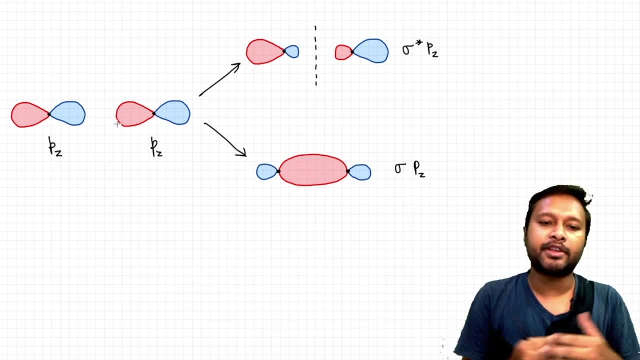 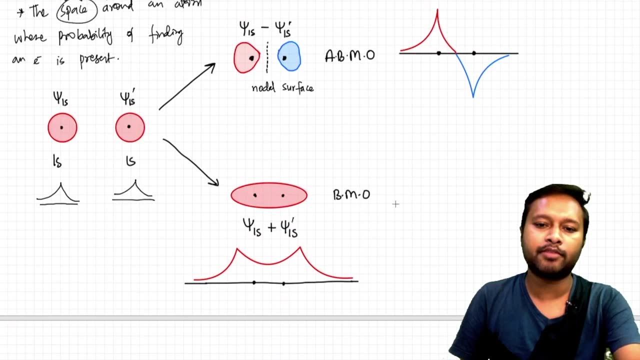 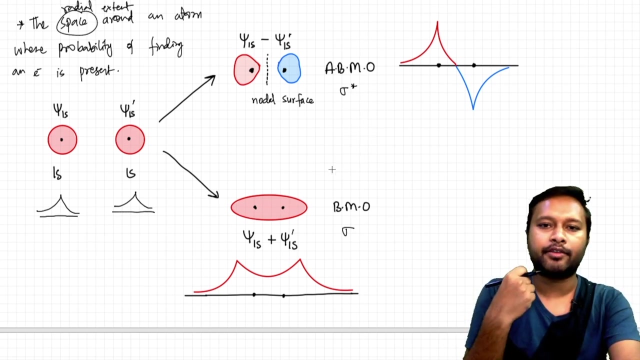 on head collision or head on head overlapping. So basically, p? z orbitals form sigma bonds. you should know that thing. And here also, these bonds which are formed will be your sigma bond only. So this is sigma bond and sigma anti-bonding. Now, if I write down the like, if I write down the parity, 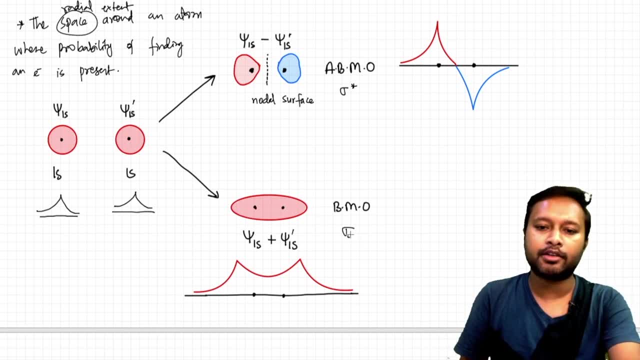 or if I write down the symmetry of these orbitals. So sigma, this bonding orbital, has a gerate parity. So sigma, this bonding orbital, has a gerate parity. So sigma, this bonding orbital, has a parity. and sigma, anti-bonding orbital, has ungerate parity because there is no inversion. 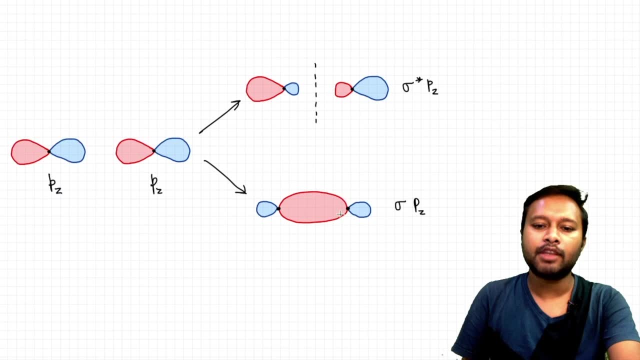 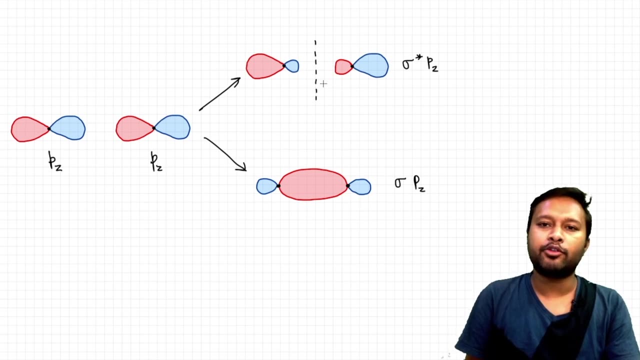 center here, whereas here you have a inversion center Now talking about your p z orbitals. So here again, these are two p z orbitals. when they are going to combine, They are going to combine in two ways: They are going to combine constructively and they are going to combine 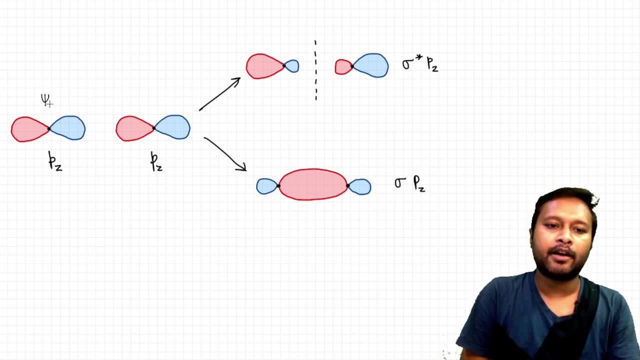 destructively. So if this is represented by psi like 2 p z, and this is like psi dash 2 p z, So here the wave form is like this: So this is like psi dash 2 p z. So here the wave form is like: 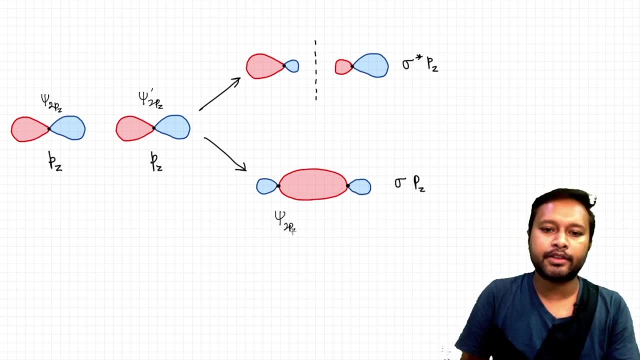 the wave function will be represented as psi 2 p z plus psi dash 2 p z, and this one is going to be represented as psi 2 p z minus psi dash 2 p z. So this is going to be the wave function. 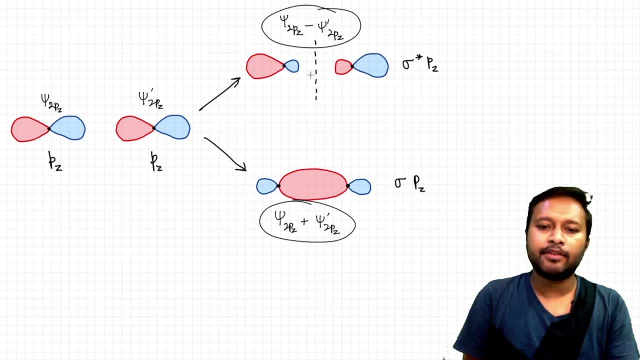 representation of these two wave functions. Now, if you see this, this is a constructive overlapping, this is destructive. So this is going to form a bonding molecular orbital. this is going to form a anti-bonding molecular orbital, the same way how we have seen for the s orbital, But here again you can see that, since there is a 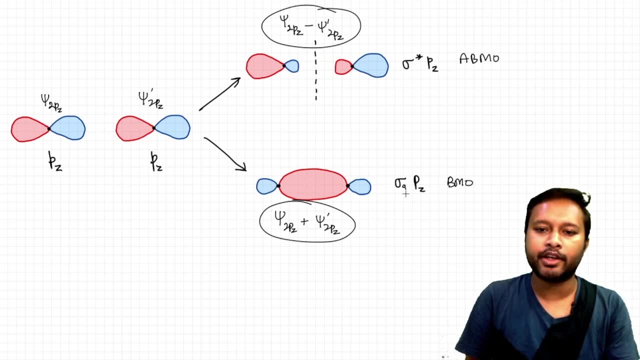 there is a inversion center in the whole thing, So the parity will be gerade. So I can write on g here. Here there is no parity because there is no inversion center present. So that is why you can write on ungerade here. So this is going to be like sigma g p z, sigma star u p z and this: 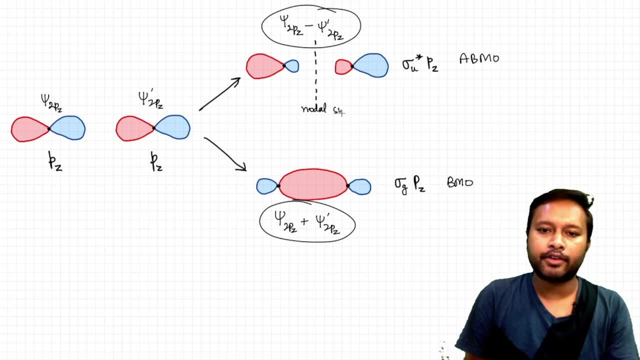 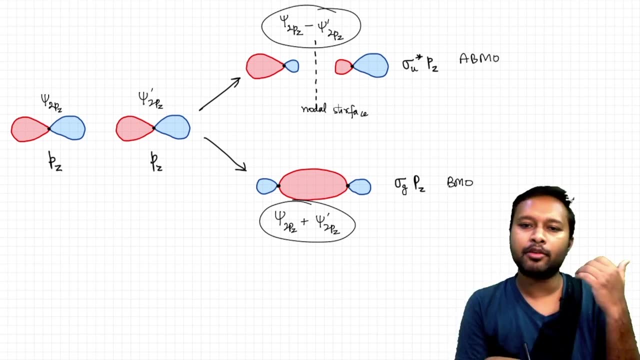 particular dotted line is again showing you the nodal surface. So simple thing it is. always, whenever there will be overlapping of atomic orbital, you are going to get bonding orbital, anti-bonding orbitals, based upon how the wave functions have overlapped. and that is what is. 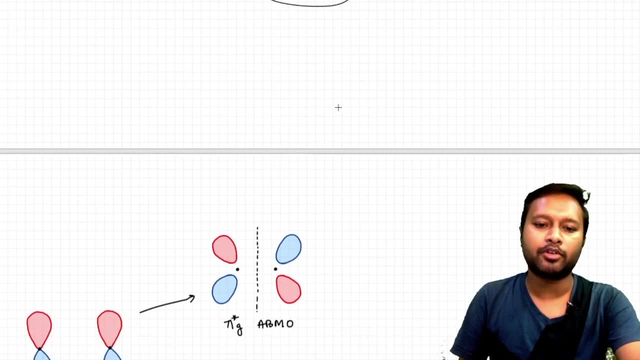 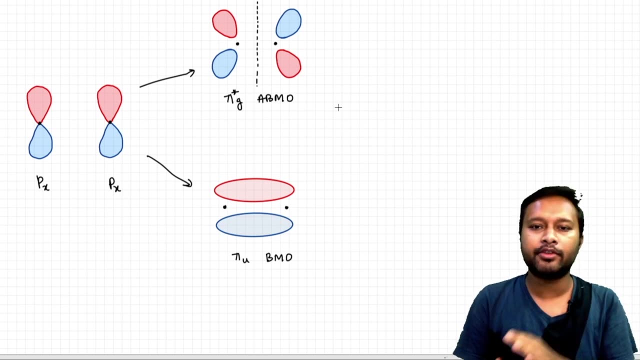 all about your linear combination. Let us understand about the pi bonds. So the pi bond can be formed by the linear combinations of your p? x orbital and of the p? y orbital. Let us say the p x orbital is the one which I have shown here. p y will also do. 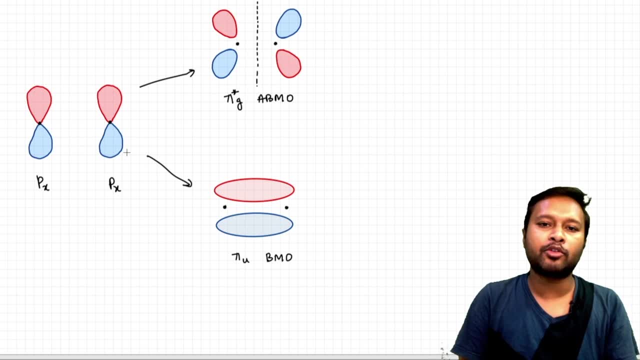 the same thing. So even the p x orbitals are going to form your bonding molecular orbital. So in that particular case, that means when they are going to do the constructive overlapping, In that particular case the wave function which you are going to get, 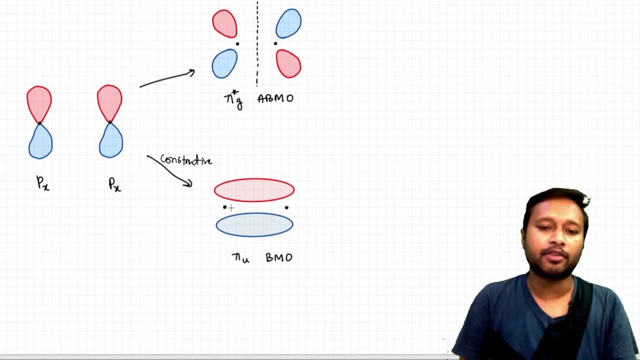 is going to be like something like this. So this is the constructive overlapping: The positive lobe are going to overlap on each other, The negative lobes are going to overlap on each other, So forming a positive cloud and a negative cloud above and below the atom. So 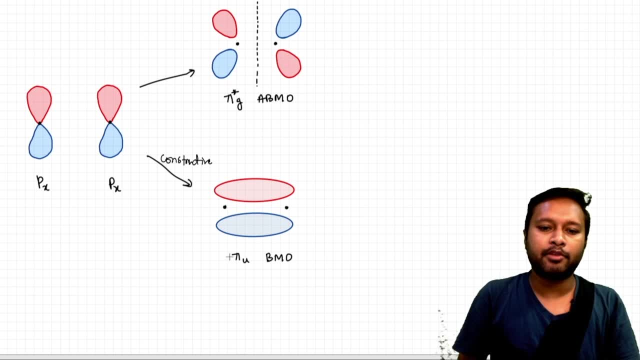 these dots are showing those atoms. Now, if you see, this will be called as pi bonding, molecular orbital. The parity of this will be ungerade because there is no inversion center, obviously here. Now, if they do the destructive overlapping, if they do the destructive, 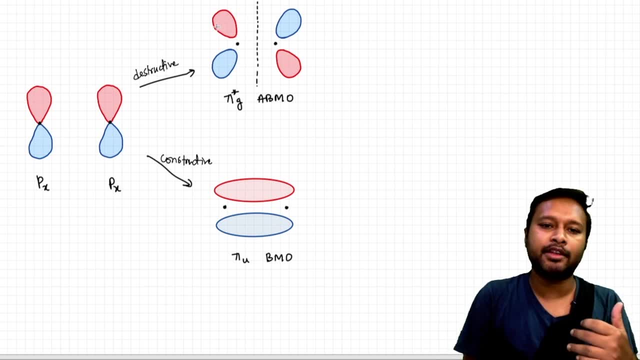 overlapping in that particular case. now, what is going to happen? that these orbitals are going to get repelled away from each other, forming a nodal plane. in this case, This is the nodal surface which we are going to get, and this particular one will be pi anti-bonding orbital. Now, 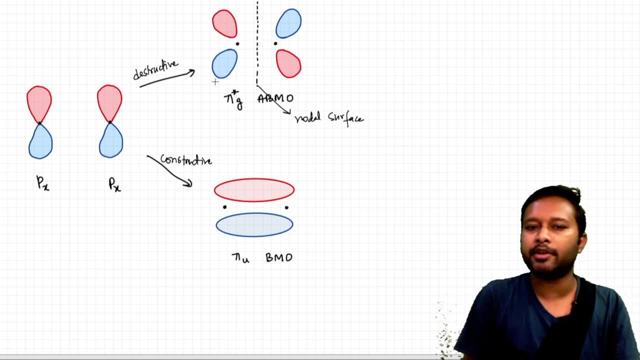 what is going to be the parity, Since, you can see, there is an inversion center, there is a point of symmetry in this case. So that is why it will have gerade as the parity or as the symmetry of this particular system or this particular molecular orbital. So we have seen three types of overlapping. How s orbitals overlap? 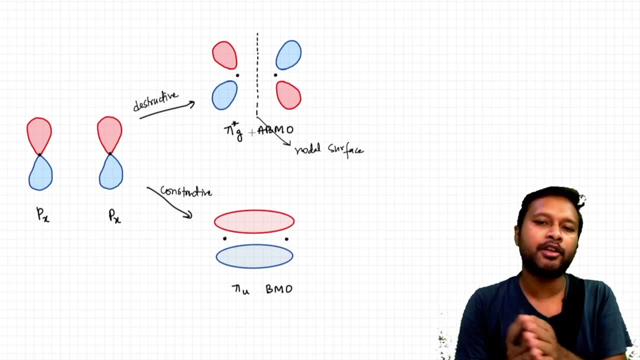 to form sigma bonding, sigma anti-bonding, How p z orbital overlap to form p z bonding and p z anti-bonding, and how p x and similarly in the same way p y will also overlap. So how p x or p y are. 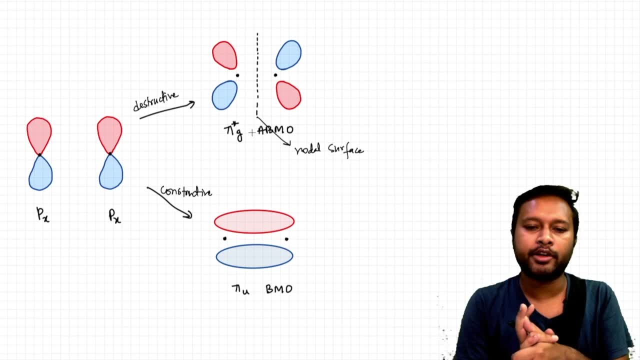 going to form pi bonding and pi anti-bonding molecular orbitals. Now, once we have understood these molecular orbital, there are certain things you should understand from the quantum mechanical point of view also. So this was all the visual representation, How visually you can understand. 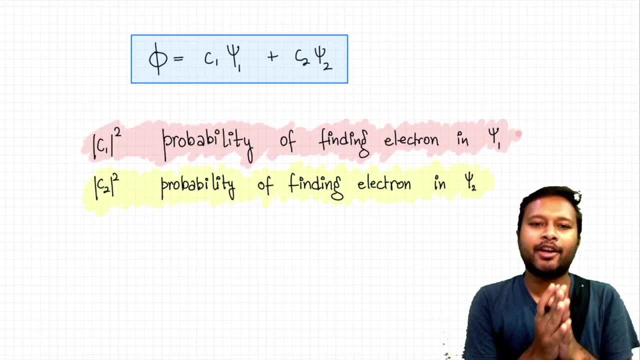 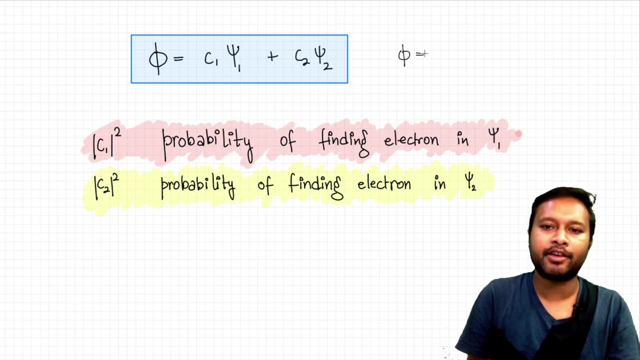 Now the time is to understand about the quantum mechanical aspect. So let us assume that we have a molecular orbital and that molecular orbital is represented as phi. So phi over here is showing you a molecular orbital. So it is a molecular orbital. So it is a molecular orbital. So it is a. 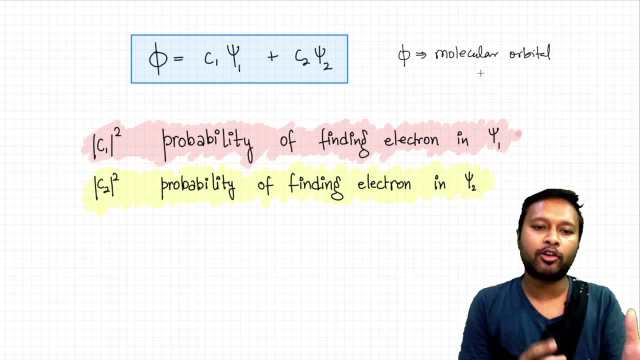 and that is formed by the linear combination of two atomic orbitals: psi 1 and psi 2.. So what are these psi 1 and psi 2?? So these are atomic orbitals. These are atomic orbitals. So what we can. 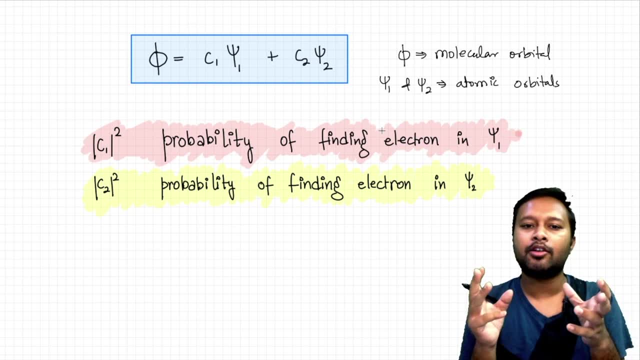 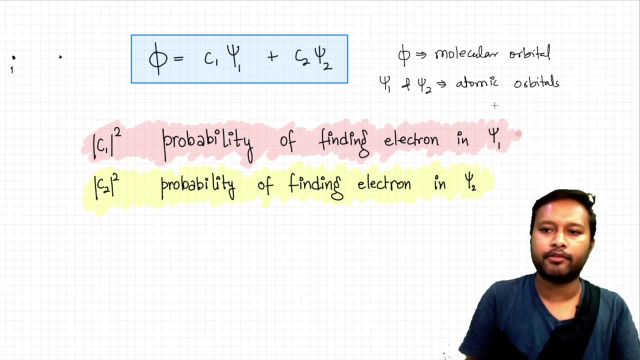 understand from here that two atoms are there, atom A or atom 1 and atom 2.. So these are the two atoms. let us say atom 1 and this is atom number 2, or I would rather draw it here. So let us say: I have. 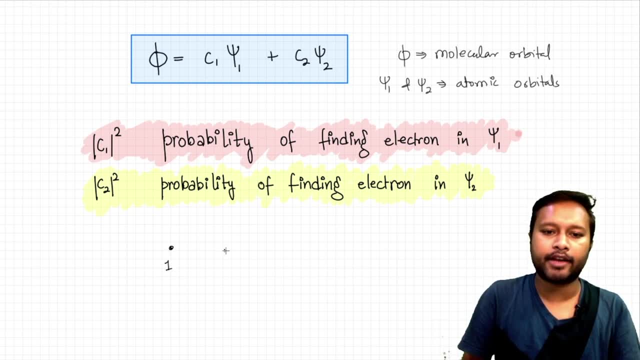 two atoms, Atom number 1 and atom number 2.. These are the two atoms. We do not know that what type of like wave function they have, whether sp or whatever orbital it has. Just we know that these two atoms are there. Both of them have certain wave function. The wave function corresponding to 1 is psi 1.. 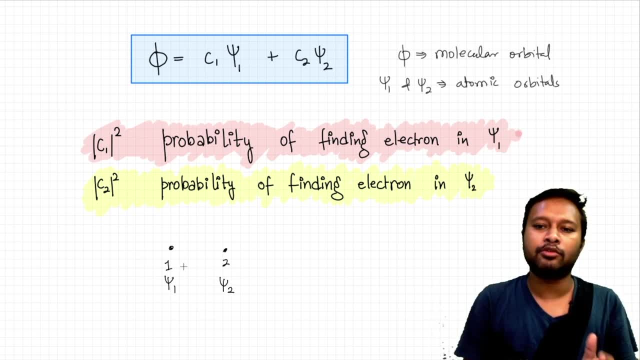 The wave function corresponding to 2 is psi 2.. When they are going to do the like, when they are going to form the molecular orbital- molecular orbital is given by your phi, So phi is representing the molecular orbital here. So when they are going to linearly combine the molecular orbital, 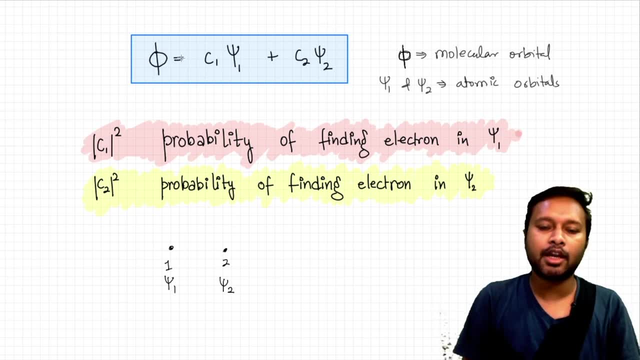 they form a molecular orbital, phi. Now this C1 and C2 comes as the coefficients of these two wave functions. like phi 1 and phi 2, will have certain coefficients: C1 and C2.. Now what this C1 and C2 tells you. So the overall wave function, or overall molecular orbital, which will be formed by 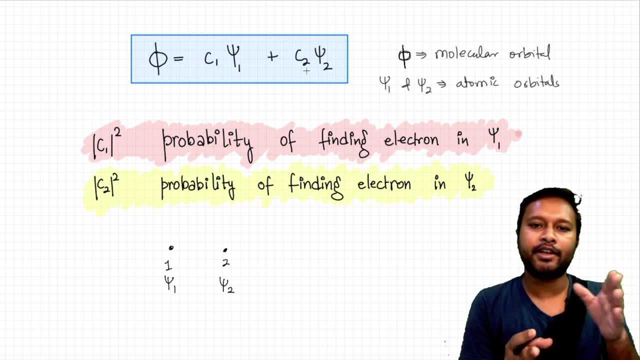 the linear combination of two atomic orbitals can be represented in this form. in the general form that phi is equals to C1 phi 1 plus C2. sorry, phi is equals to C1 psi 1 plus C2 phi 1.. So this is. 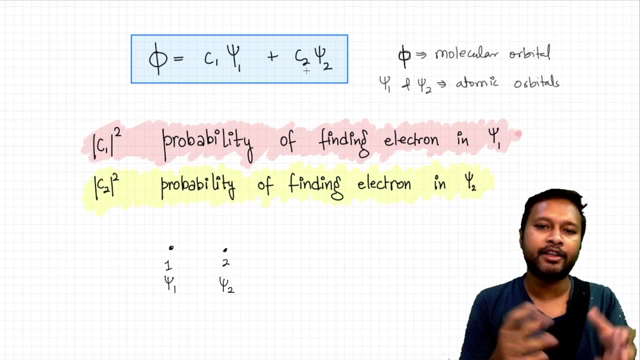 C2, psi 2.. So just understand this: that wherever you will be getting linear combination of linear combination of atomic orbital, the molecular orbital will be represented like this. So here two atoms have linearly combined. It may be possible that there are more than three atoms. 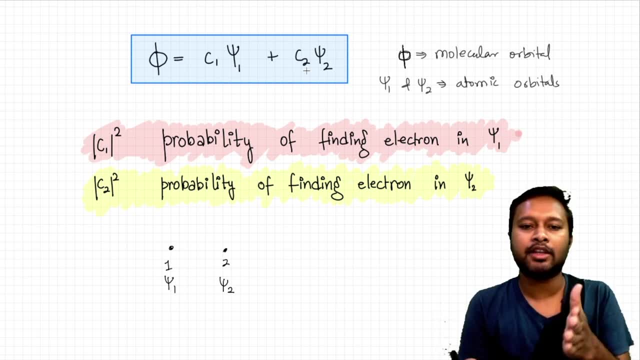 which linearly combine. So in that case we will have more wave functions there, If three will be there. so C1 phi 1 plus C2 phi 2 plus C3 phi 3.. That is how it will be. So C1, C2 and C3, or C1- C2. 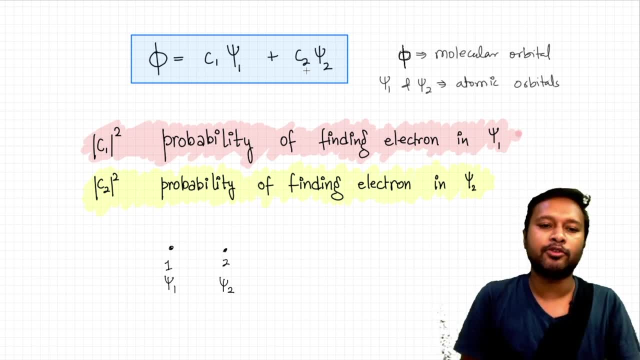 over here are basically the coefficients. So what these coefficients tell you? So these coefficients, the square, the mod of the square of coefficients, tells you about the probability of finding electron in that particular orbital or that particular wave function. So what is the probability that C, These two atoms are going to share electrons to form the bond? 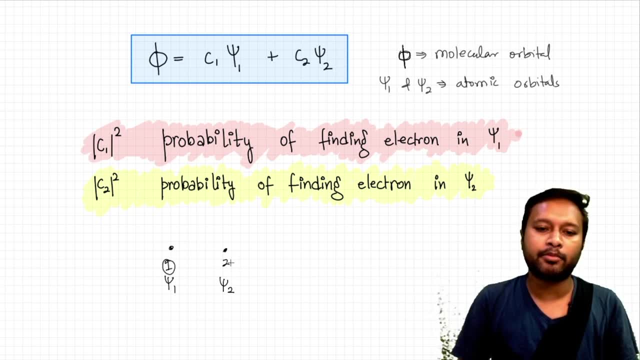 between them. Obviously, this atom A first and atom number two. both are going to share electron to form the bond between them. Now what is going to happen that? What is the probability? Now, it depends upon the probability that C1 phi 1 plus C2 phi 2.. So what is the probability that C1 phi 1? 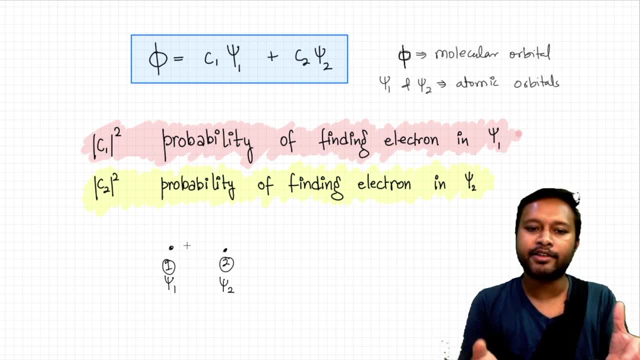 plus C2 phi 2 becomes the coin of C minus than C. Let us now Мыukan-Zga celebrated Episode 8. The analysis given by Dr arrogance told that of oxygen atoms thing, this C2 phi is C and C3 phi 2 is C1 magnimax. 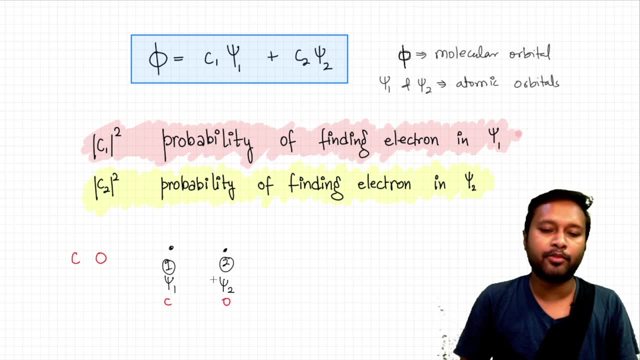 If C is negative, so this way it is: tenha probably equal to 0.4, or 0.5 plus 0.5, maybe. so. So to proof that we have now ваши signalsиты, czo do babμr hebben. so let us say, if C0, wh, covidやn, there's something belong one electron of the key molecule, soозweil, понys think, combined in the BPM, how this electron is going to get distributed among them, depending upon the dipole moment of the atoms, or depending on the dipol moment to the molecule, or they are different factors. So let us say that we have a carbon dioxide molecule, okay, co molecule, financialwarzschild. 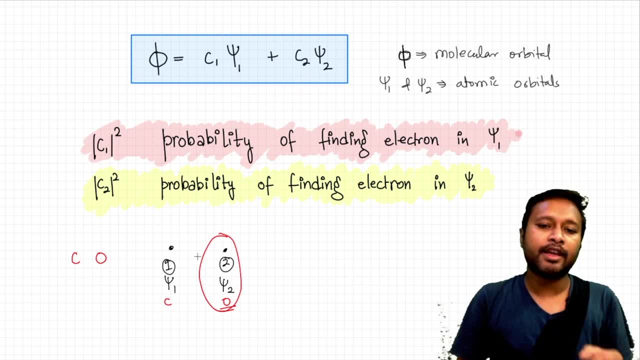 electronegativity of the oxygen atom. So in that case, probability of finding electron in the psi 2- that means the wave function corresponding to oxygen- will be high as compared to the like probability of finding electron towards carbon side. So in that case, what will happen? 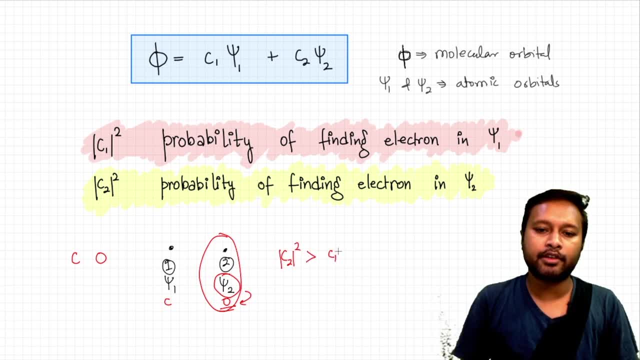 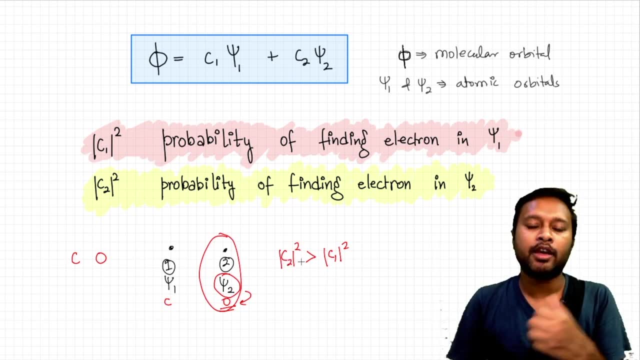 that C2 square will be greater than C1 square. So what does it tells you that the probability of finding electron around the second atom is more as compared to the probability of finding electron around the first atom. So this tells about the dipole moment of the molecule, and all. 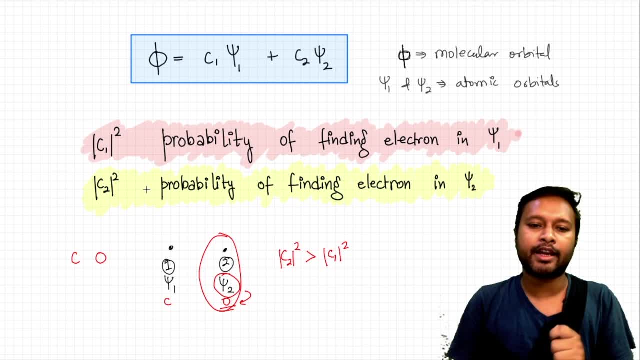 So yeah, C1 square and C2 square gives you a very important property. that means it tells you about the probability of finding electron around that particular like atom. Now there will be different questions. I will take them and I will show you they were asked in gate exam and how to solve them. 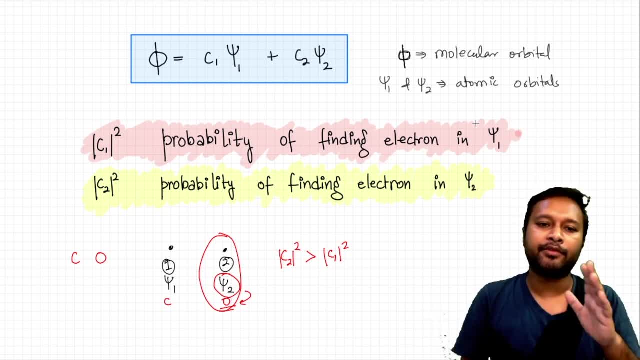 based upon the same concept. So make this thing very clear: that if you are given with a molecular orbital where you have linear combination of different atomic orbitals, So the coefficient of those atomic orbitals is going to be greater than the probability of finding electron around. 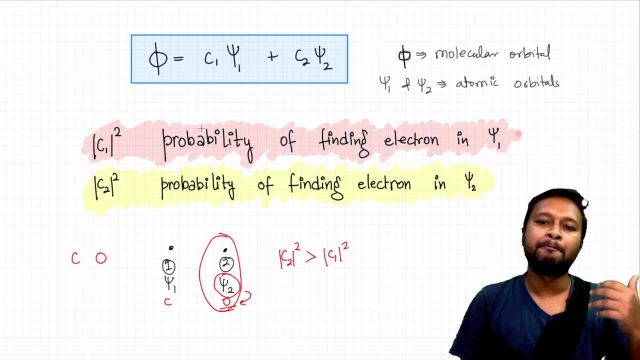 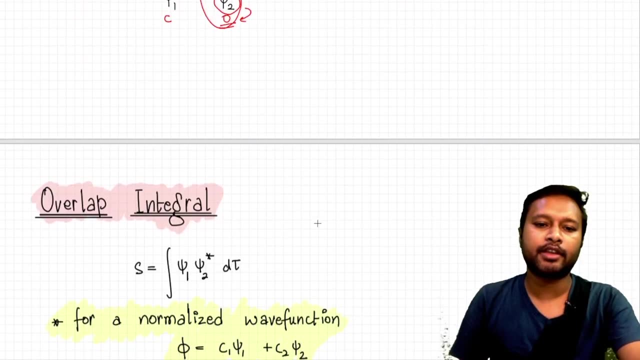 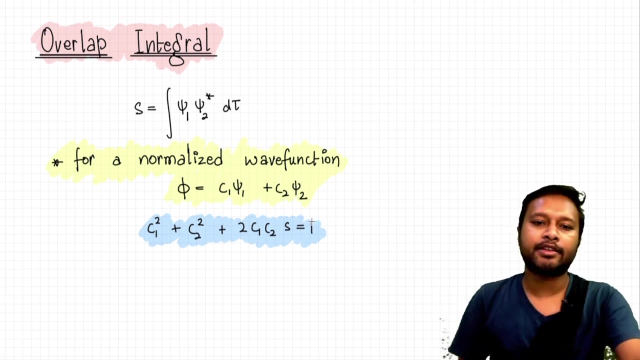 that particular atomic orbital Square, of coefficient of those atomic orbitals, tells you about the probability of finding electron around that particular atomic orbital. Now, once you have understood this thing, the next thing is even more interesting, and that is your overlap integral. Now, what does this overlap integral means? It means in the starting, as I told you, that the atomic 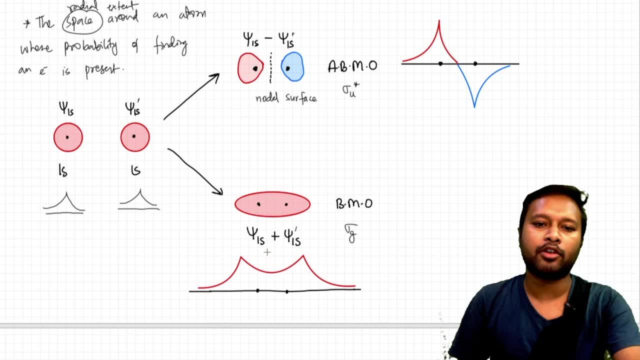 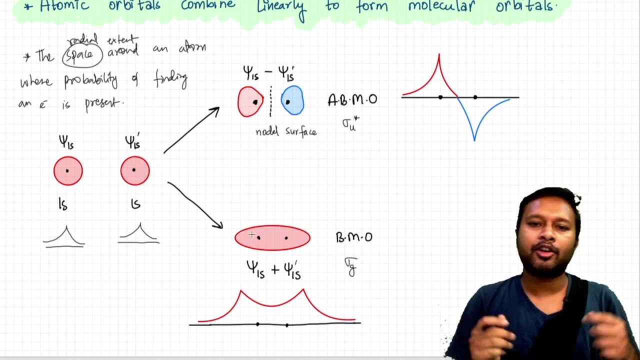 orbitals overlap to form bonding and anti-bonding orbital. let us look upon this example. So these were the wave functions which overlap and they formed these bonding and anti-bonding molecular. now the question is that: how much do they overlap? okay, how much overlapping is between? 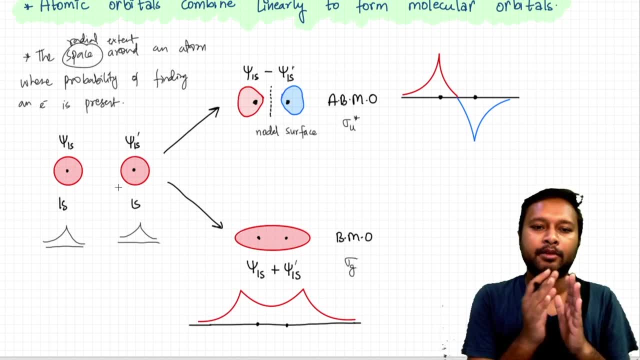 these two atoms, so that overlapping, that amount of overlapping, will be discussed by the overlap integral. so overlap integral tells you that whether there is overlapping happening or not happening, for example for the bonding molecular orbital, you can see that yes, there is a overlapping happening, like they are actually going to overlap. so this is actually how it is going to be and 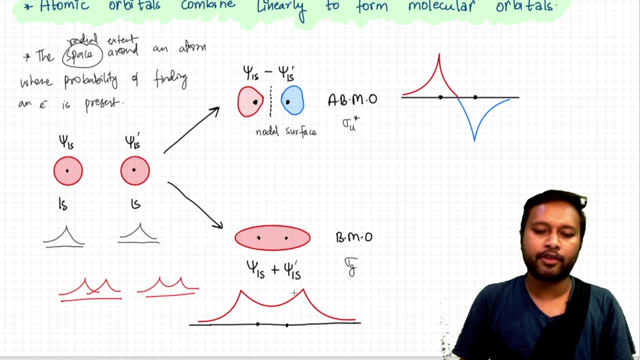 then the overall wave function will look something like this: right, that's what you have seen here. so there have been certain amount of overlapping, which has happened. so how much overlapping has happened? that will tell you that how much strongly they have bound or how much close those atoms are. 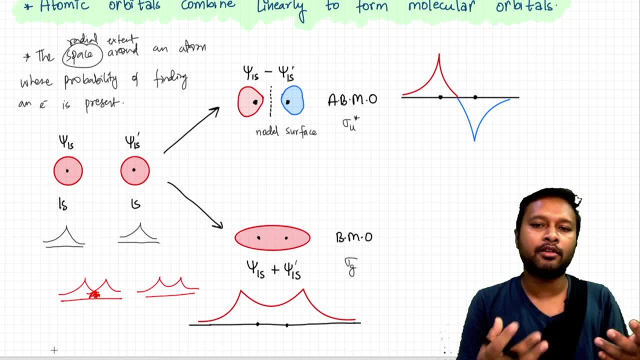 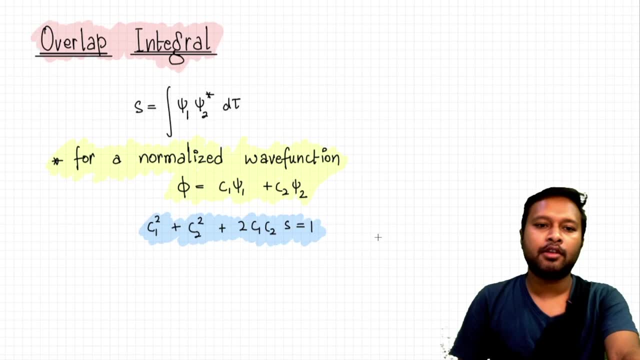 so these all parameters, or these all values, or these all like properties you are going to get from the overlap integral. so overlap integral becomes a very important concept once again. so the overlap integral is denoted by s and s is equals to integral of psi one, psi two, star d tau, where psi one and psi two belongs to the wave function of the two atoms. as 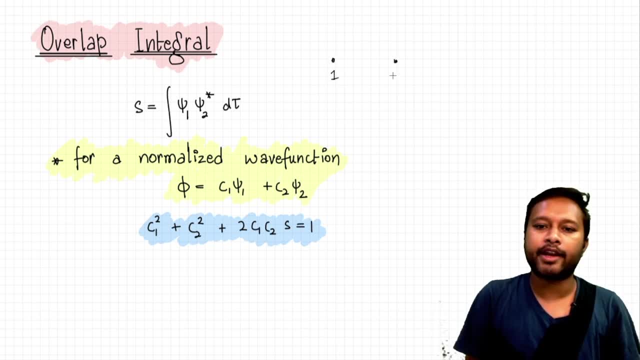 we have discussed. so if there are two atoms, atom number one and atom number two, so the wave function corresponding to this is psi one. corresponding to this is psi two. now, if they overlap, so how much they have overlapped, that will be calculated by the overlap integral, and this will be psi one, psi. 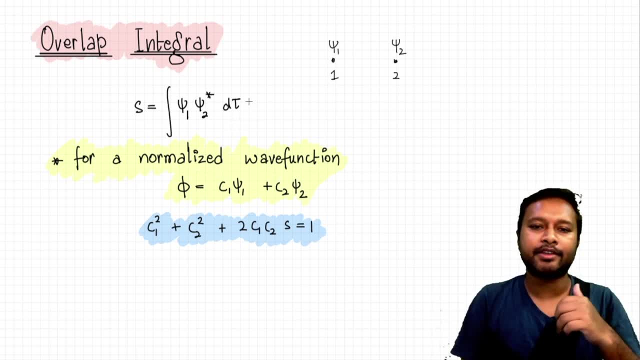 two star d tau. okay, if it is in one dimension, d tau will become dx. if it is a spherical, then d tau will have different value. so it depends upon that. now for a normal, normalized wave function. if you are given with a normalized wave function, let's say this is how we. 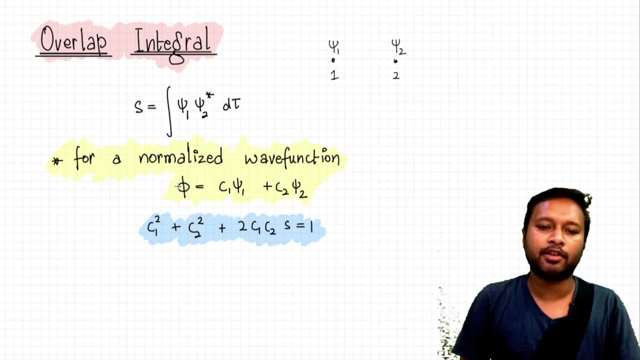 have taken one more example, like once again, we have taken the similar example of the molecular orbital wave function. so phi is equal to c 1, phi 1 plus c 2, phi 2. so for that overlap integral can be calculated from this formula. we say c 1 square plus c 2 square plus 2, c 1, c 2 s is equals to 0. 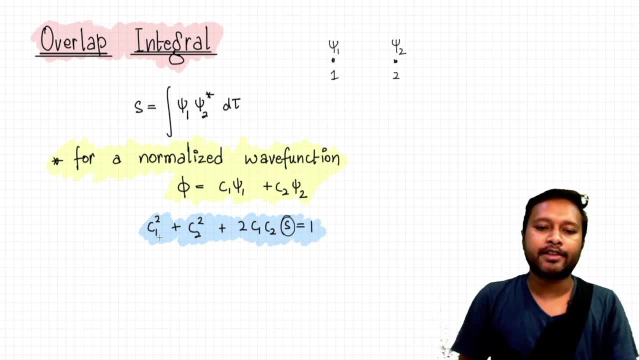 where s is basically your overlap integral and c 1, c 2 are basically your like coefficients of your like atomic orbitals in the molecular wave function. so this much knowledge if you have, if you understand what the wave function is, how the atomic orbital overlaps, like what is going to be. 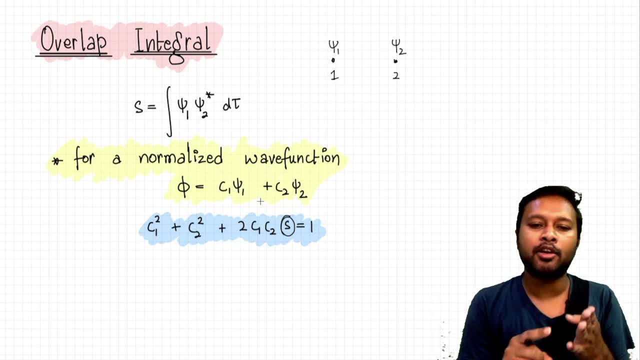 the overlap integral, or what a overlap integral tells you about? what does the coefficient of the atomic orbital tells you in a molecular orbital? if you know this much, at least you can do one type of quotient from quantum mechanics, and this is going to be very useful if you are doing a quotient from. 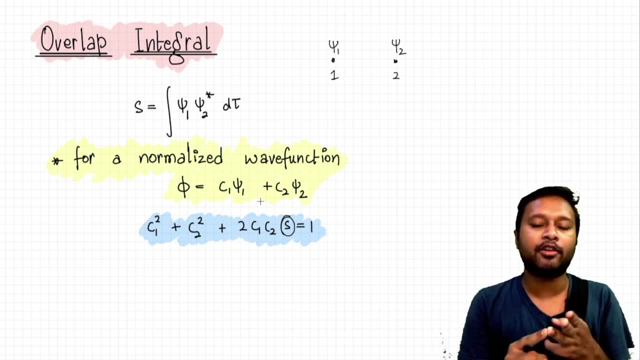 iit jam if you are doing a quotient from a cs ironet or you are doing a quotient from a quantum or if you are doing a quotient from your gate exam also. so in any competitive exam this is the easiest type of quotient which can be asked, based upon chemical bonding and coordination. sorry. 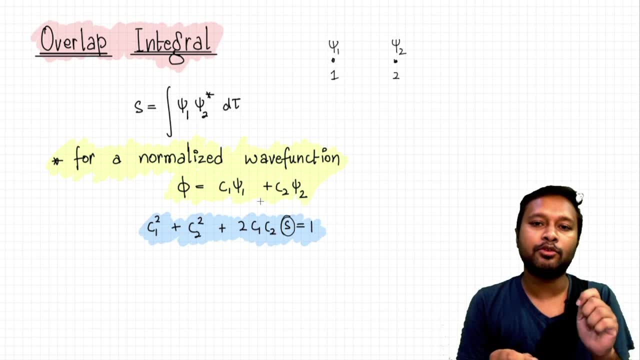 chemical bonding and quantum chemistry collectively. okay, so you should be aware about it. if you are not aware about it, just let me know in the comment that, yes, you got to know this from this particular video. all right, so let's take some questions now from the previous years of gate exam. let's try to 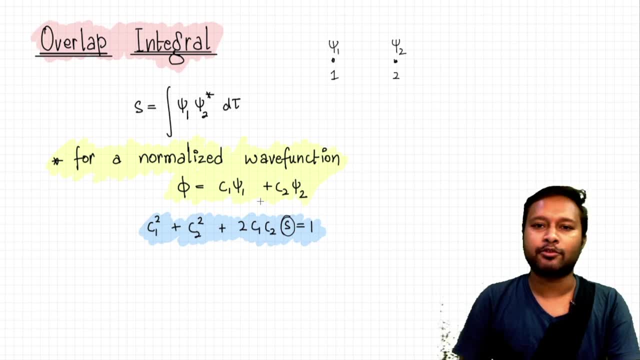 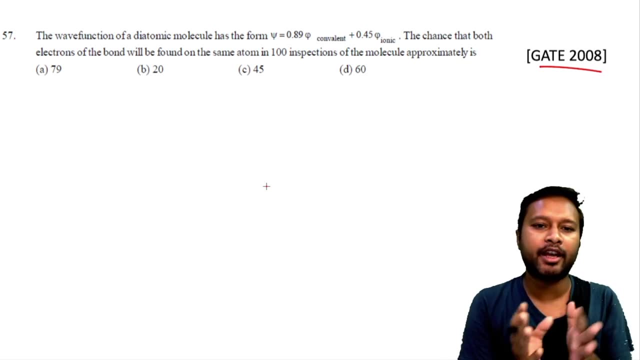 solve them out and see how these concepts will be used to solve those questions. all right, guys, we'll start from this particular question, which was in gate 2008 exam. and the quotient says that the wave function of a diatomic molecule has the form. the wave function is given to you as psi is equals to 0.895, covalent okay, and plus 0.45. 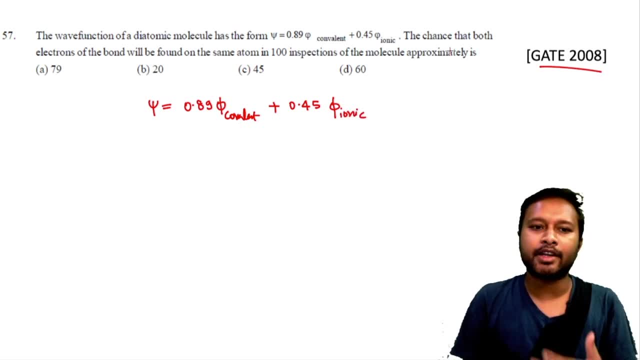 phi ionic. okay, now it says that the chance that both the electron of the bond will be found on on the same atom. so both the electrons of the bond will be found on the same atom in the hundred inspection of the molecule, approximately. so they have tried to confuse you a little bit, but you have to stick. 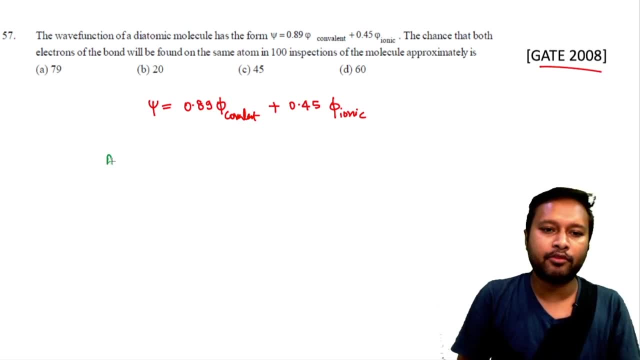 to the concept. okay, so you remember, when out there are two atoms, a and b, and when a covalent bond is formed, so basically electrons are being shared with both of them. so if i draw the lewis structure of of a molecule, a, b, so what will happen? that a will have electron, b will have electrons. so 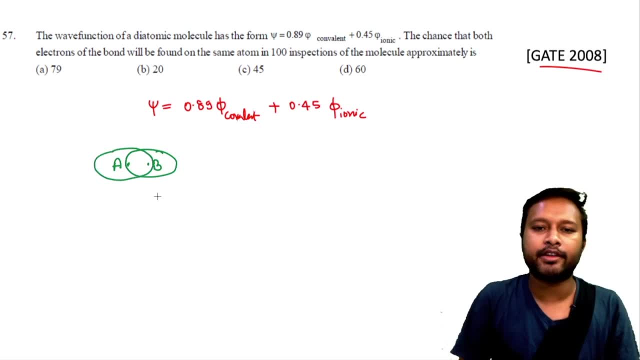 the lewis dot structure is basically made like this. okay, so these electrons are shared between both of them. but when an ionic bond is made, or when an ionic compound is made, let's say that b is more electronegative than a. so what happens? that a give its electrons to the b atom? 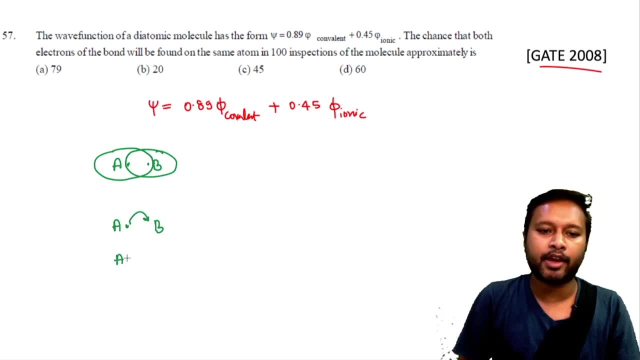 okay, so it gives its electron to the b atom and that's how happens that a will have plus charge and b gains two electrons along with the negative charge. so that's how the ionic bond is made between them. so ionic bond happens, or ionic bond is made when the both, the electron, stays on a single atom. 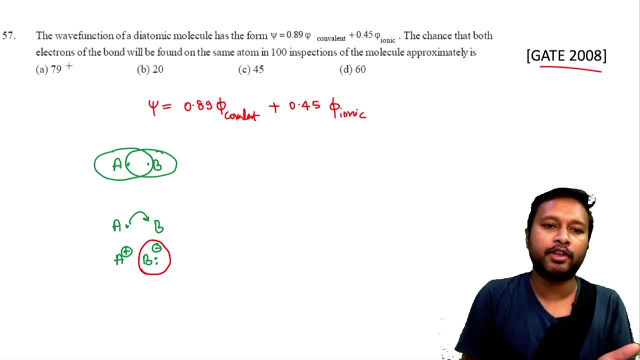 and that's what is asked in the question. it says that the chance that both the electrons of the bond will be found on the same atom, so if both the atoms or both the electrons are being found on the same atom. so basically they are talking about the ionic bond. so you, 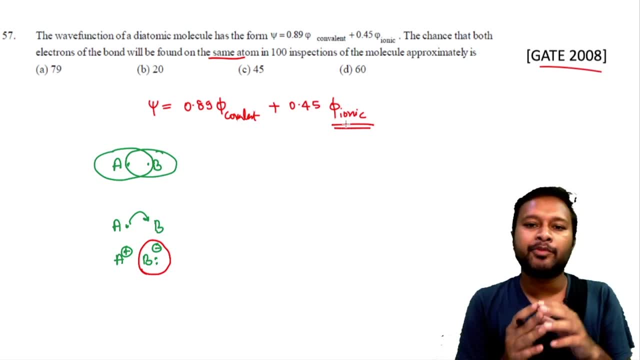 just have to look upon the ionic part of the wave function. now they are asking the chance or the probability. right, chance means probability, so how you will get the probability. so that is going to be the coefficient now, since the coefficient is 0.45, and i told you that. 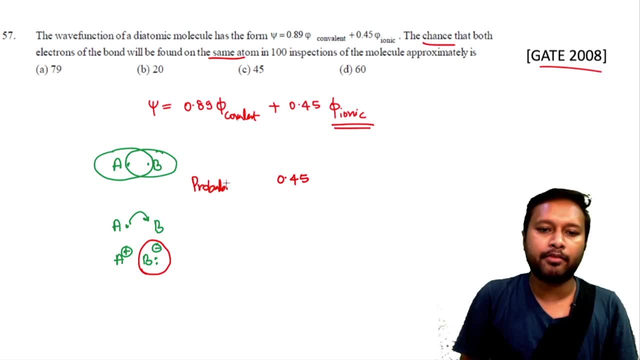 the probability. i'll just write down here that the probability basically tells you the square of this. okay, so mod square of this. so just square this up and if you square you will get 0.2025. you can use your calculator because it's a gate exam. now they are asking in the 100 inspection. 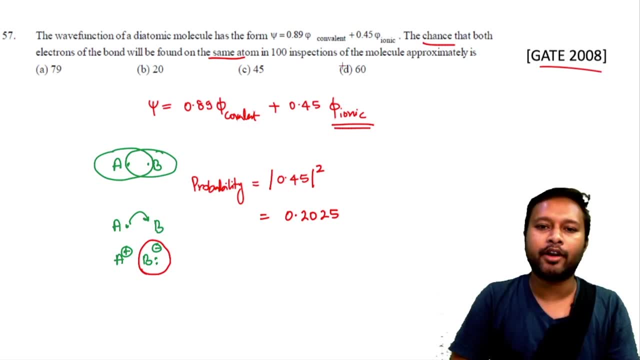 that means you have to take it to the terms of 100 or you have to come multiply it with 100 to get in the form of 100 inspections. okay, so 0.2025. just multiply it with 100 and you are going to get 20.25. that means the correct answer is option number b, which is around: 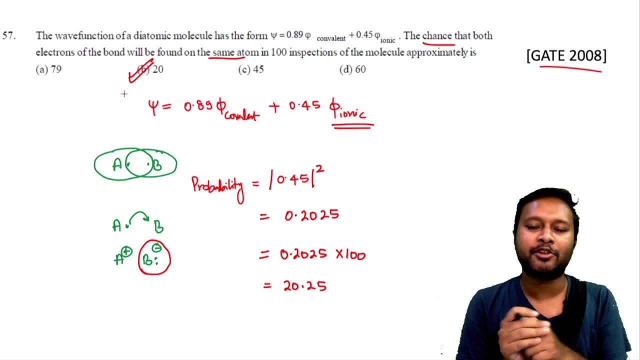 20.. so, approximately, the correct option comes out to be option number b. so see how simply the question was a little complicated, but how simply you have applied whatever you have studied to solve this question. you just need to know the basic idea of ionic and covalent bond. let's go. 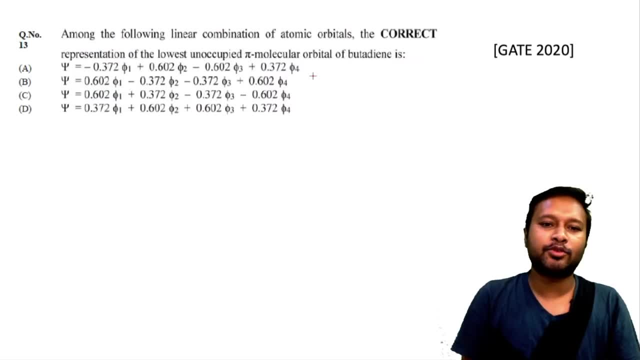 for the next question, then okay, the next question here is pretty simple. this type of questions are generally done on a very simple concept. let's go for the next question then. okay, the next question here is pretty simple. this type of questions are generally done on a very simple concept. 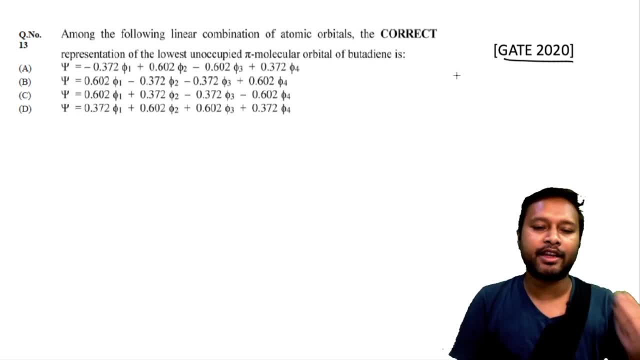 okay, it says this was first of all asked in gate 2020, that means very recently, and it says that among the following: linear combination of atomic orbital, the correct representation of lowest on unoccupied pi, molecular orbital of butadiene. now for this you need to know. 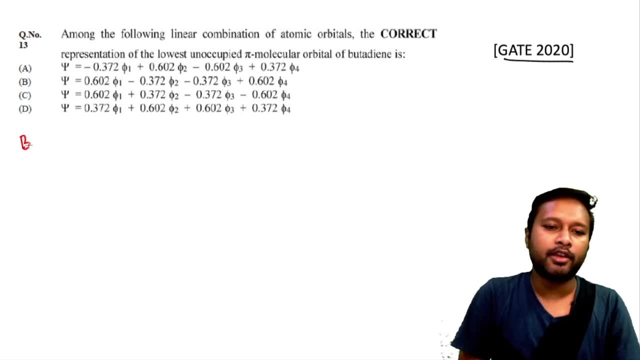 some basic understanding of butadiene first of all. okay, so butadiene, what it is. this is basically your ch2, double bond ch, single bond ch and double bond ch2. this is your butadiene. there are four atoms. we are just talking about the pi orbitals here, because this talks about the pi molecular orbital. 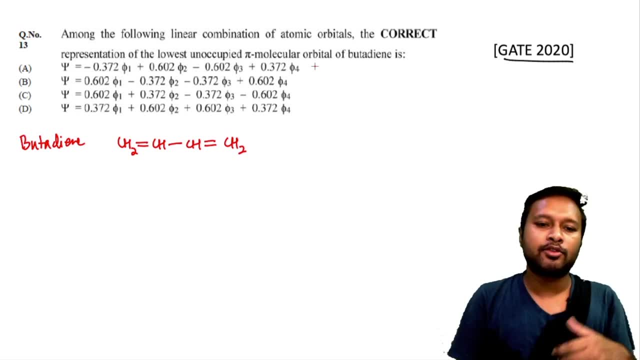 so there will be four atoms which contain pi orbitals. so you will have four molecular orbitals, four pi molecular orbitals. so those will be given as your psi 1, psi 2, psi 3 and psi 4.. you can draw them, even the orbitals you can draw. but okay, fine, we'll try to draw it. so basically, what concept you? 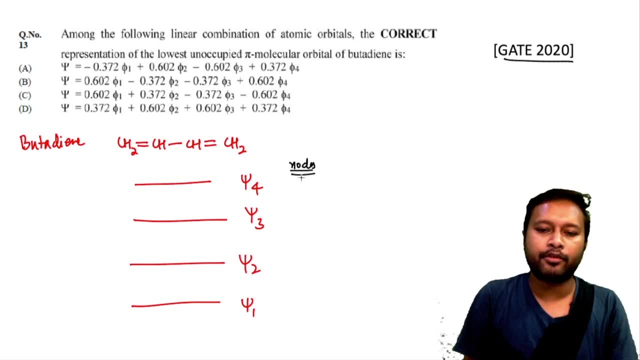 have to apply is number of nodes. okay, so if i write down the number of nodes here, so the number of node is one less than which orbital you are talking about. so psi 1 will have 1 minus 1, that is 0 nodes. psi 2 will have 2 minus 1, that is 1 node. psi 3 will have 3 minus 1, that is 2 nodes. 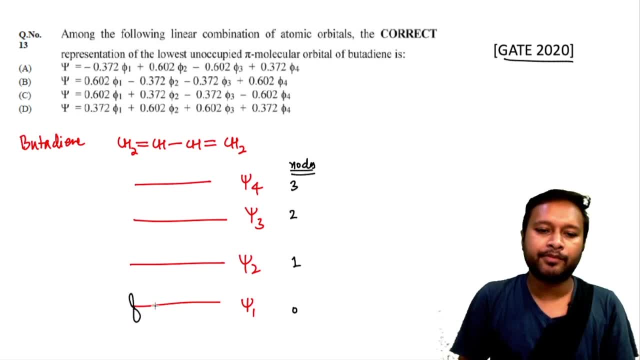 and psi 4 will have 3 nodes. so if i draw the wave function, so this is how it will be okay- the four orbitals will be here. the shaded part is showing you the positive part, then unshaded is the negative part. so 0 nodes in this case. in this case you will have a single node. 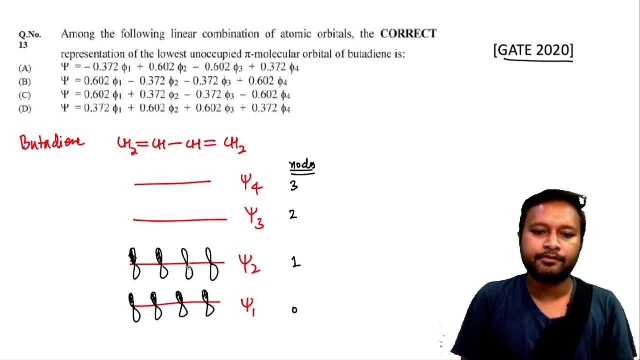 so that means it will be drawn something like this: okay, the wave function will be something like this: for psi 3, you have two nodes, so you can draw those two nodes like this. okay, where those nodes are, i'll explain you that also. okay, so in this case the node is here, in this case the nodes are. 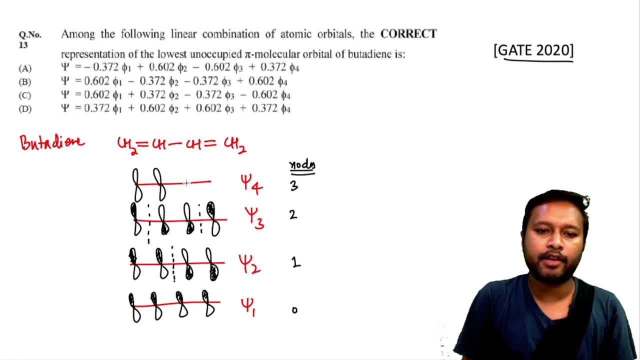 in these two places. psi 4 will have three nodes, so that means one, two, three and four orbitals. so the are here. okay, this is how you will make, and it will have one node, two node and three node, okay, so all the three nodes are here now. once you have understood this much, it's pretty simple to 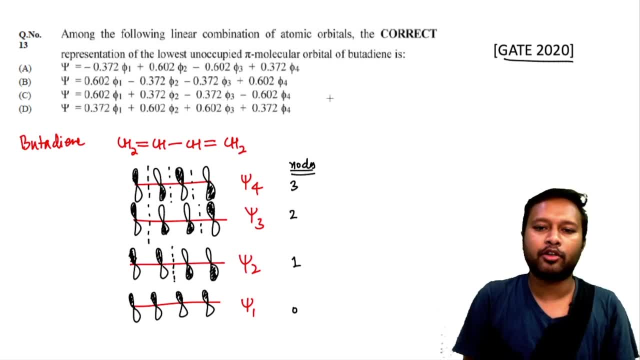 approach the question. they are asking about the lowest unoccupied molecular orbital, so they are talking about lumo. so you should know about homo and lumo. so how many pi will electrons are there? so 2 and 2 that means 4 pi electrons. so if i fill those pi electrons in these energy levels, so they 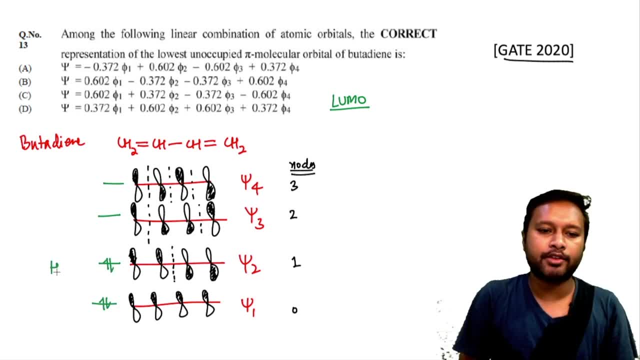 will be filled according to the houns rule, like this: making this psi 2 as your homo, because it is highest occupied molecular orbital, and your psi 3 as your lumo. okay, now psi 3 will be your lumo, and how many node it has? it has two node. now you have to look upon the options where you have two nodes. 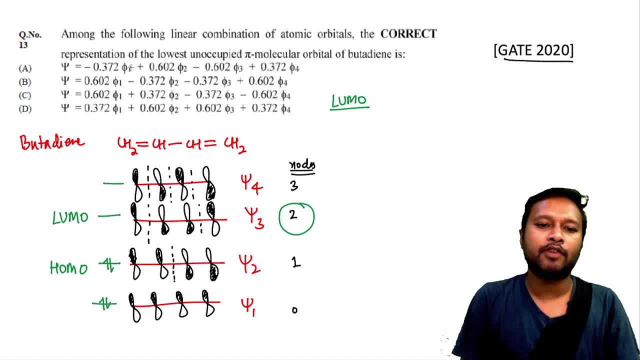 present, okay, so if you have to check out the nodes here, so just you have to see that how many times the sign is changing. in option number eight the sign is changing once, okay, from here to here, once and then again thrice. so how many nodes? you have three nodes in option number a. for option number 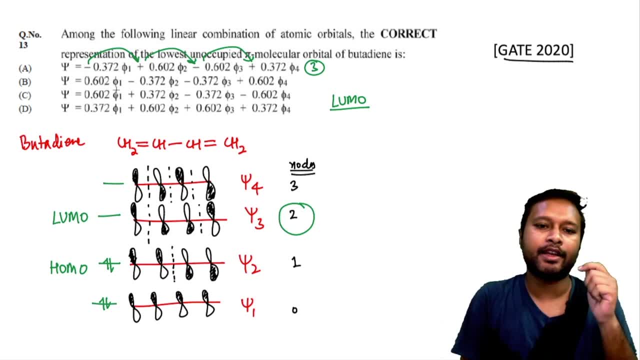 b. you can see that sign is plus here. so plus to minus sign has changed once. it has not changed yet, but it changed here. so there are two nodes here. two times the sign has changed from plus to minus. it remained minus, but here again from minus to plus. so one, okay, one from here to here and the 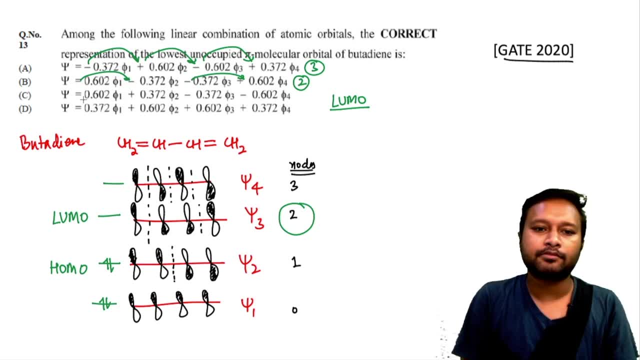 other time from here to here. so two nodes. option number c: see it is plus, it is also plus, so no change. the only change it happened is the change in the reason. it changed in the reason, the change. just one, so just one node, in this case in option number d, since all of them are plus, so zero nodes. 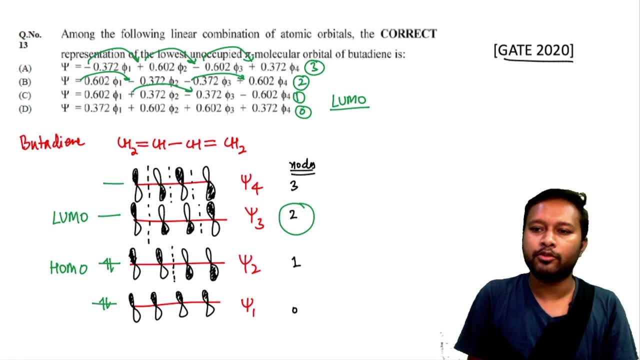 in this case. so you are talking about your lumo. lumo is going to be your psi 3. that means two nodes. so two nodes is in option number b. option b becomes your correct answer. so just by understanding the nodes and just by understanding, just by finding out the number of nodes, you can simply 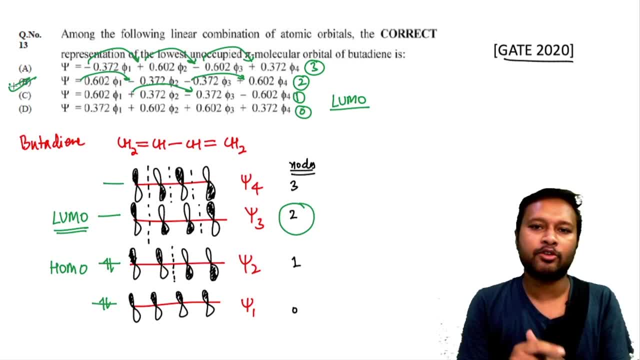 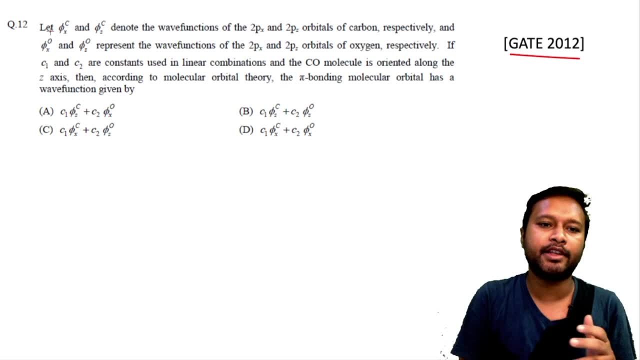 answer, you don't have to worry about the coefficients as well. okay, so this is how you have to do this question. all right, let's go for the next one then. all right, so let's talk about this question, which was asked in gate 2012 exam. it says: let phi x c and phi z c denote the wave. 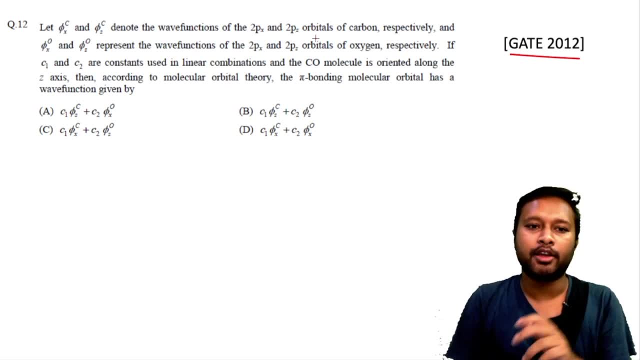 function of 2 px and 2 pz orbital of carbon. okay, so understand this. this phi x c denotes x orbital of carbon. this c is denoting carbon, x is denoting the x orbital, like this is denoting the 2 px orbital of carbon. you have to do this question, all right, so let's go for the next one then. all right, so let's talk. 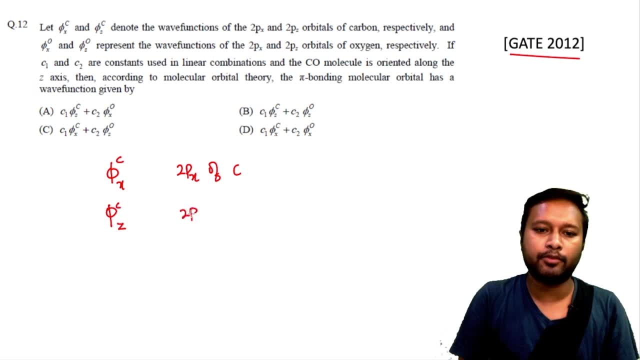 in gate 12, so let's talk about the next question. all right, so let's go for the next one then. all right, so let's talk phi c z is representing 2p z- orbital of carbon. okay, this z is representing that. it is 2p z. 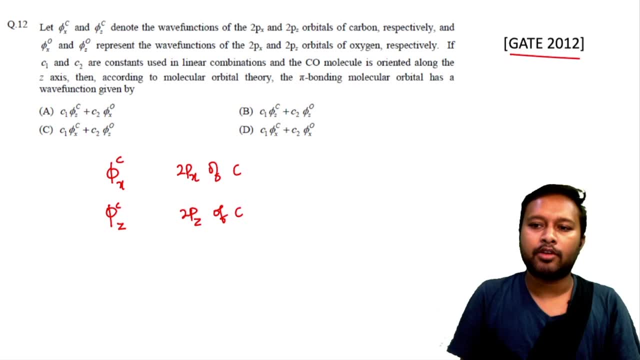 this c is representing that it belongs to carbon. now, if you take the other part, that is phi x o, so i can write it down as phi x o. this represent the 2p x orbital of oxygen and phi o z represents 2p z orbital. 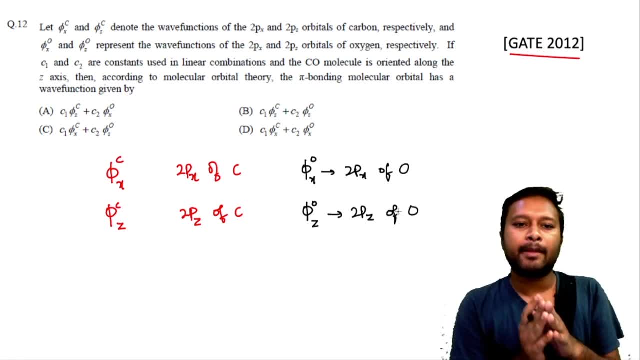 orbital of oxygen. Now they are asking where C1 and C2 are the constants used for the linear combination. the carbon monoxide or the CO molecule is oriented along the z-axis. So CO molecule is oriented along the z-axis Then, according to the molecular orbital theory, 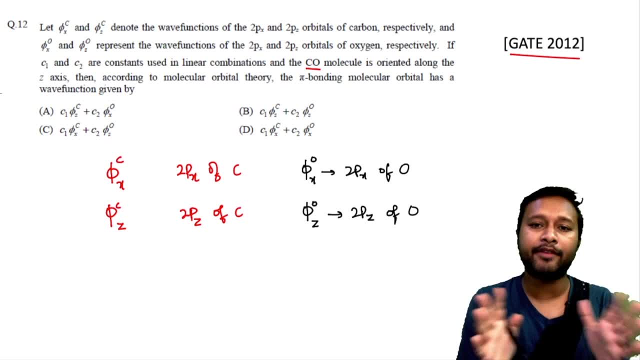 the pi bonding molecular orbital have a wave function. So you have to just understand this: that if carbon monoxide is getting formed and if it is oriented along the z-axis, this is, let us say, the z-axis, So where does the other axis goes? So let me just write down: 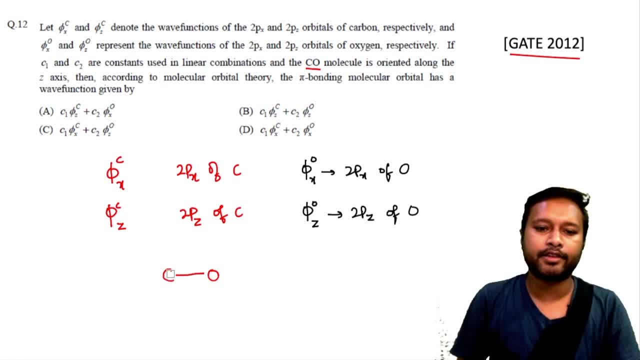 it properly. So, or shall I? I shall make the axis system to explain. So let us say that the three-axis system is like this: You have the z-axis, you have x-axis and you have y-axis. So this is x-axis, this is z-axis. Now the carbon monoxide molecule is oriented along the 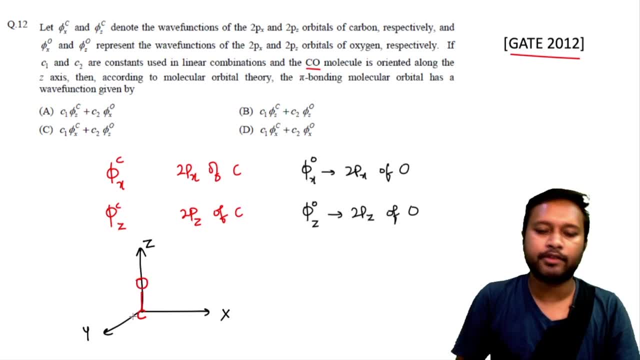 z-axis. So carbon is there and here you have oxygen. So this is how the carbon monoxide orbital is. Now, which orbitals will be involved in the sigma bonding? So, obviously, those orbitals which are along the z-axis. So which orbitals will be involved in the 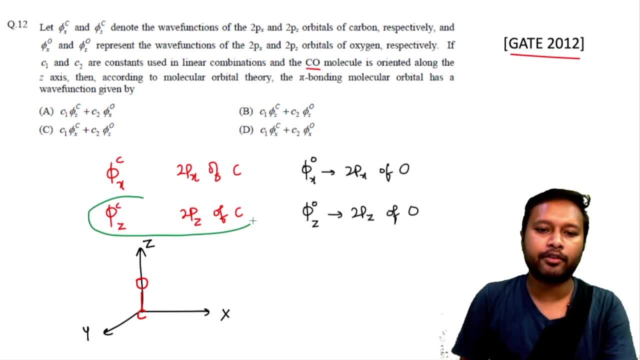 sigma bonding. It is pretty simple to understand. The z-orbital of carbon and the z-orbital of oxygen will be involved in the sigma bonding. They will combine to form the sigma bond. Now, which orbitals are involved are going to be involved in the pi bonding, So 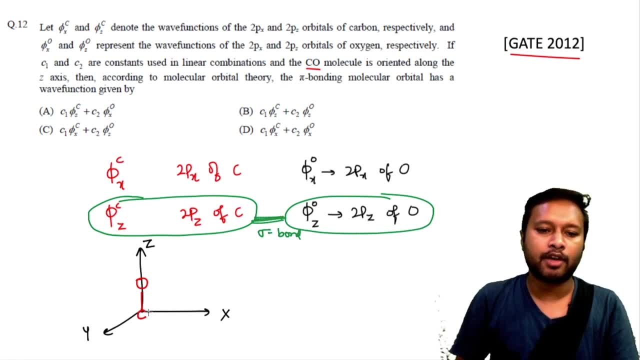 obviously, if I draw the orbitals here. So carbon pi orbitals will be like this, and oxygen also. The pi orbitals are always present perpendicular to the plane, So this is how the bonding is going to happen. So which orbitals will be involved in? 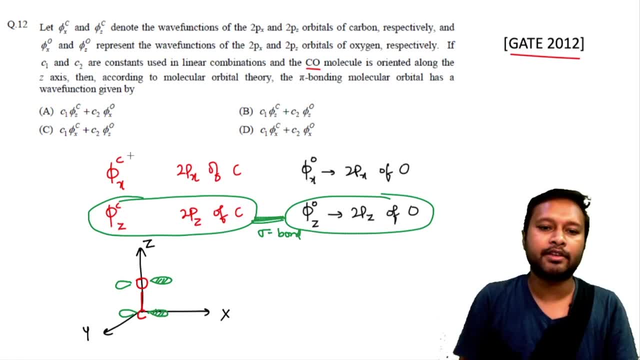 bonding. So the orbitals aligned along the z-axis, That means 2p, sorry. the orbitals aligned along the x-axis. So which orbitals are those? Those are your 2px and 2px of your oxygen. 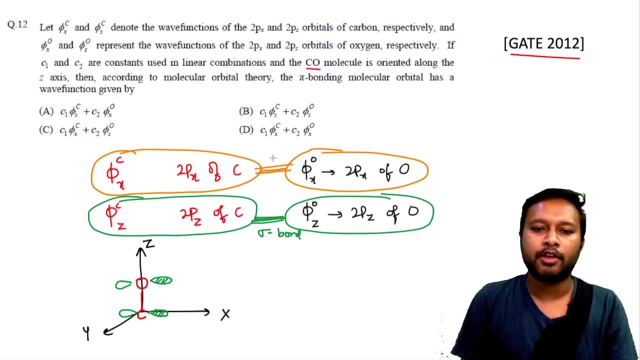 So how the bonding is going to get formed or how your. so this is going to involve in the pi bonding. So what is going to be the answer? So the pi molecular orbital will be represented as, like: if I call it as phi, let us say phi pi, that is phi, bonding molecular. 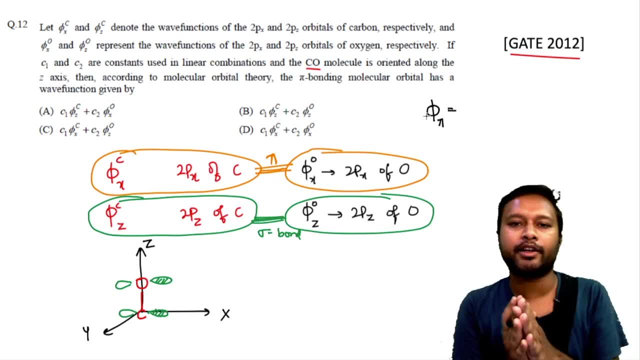 orbital Bonding. that means that has to be constructive overlapping. We are talking about pi bonding, molecular orbital, not anti-bonding. So for bonding the sign should be plus. Obviously the answers are: having plus signs You do not have to worry about. but if they confuse, 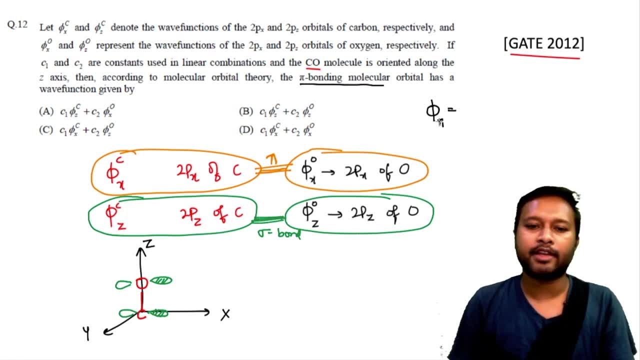 you with the sign. you should know that bonding molecular orbital will have a plus sign. Which orbitals will be there? So obviously c1. you will write down, because that is a linear combination coefficient. So let us write down c1. and then which orbital? So phi, xc, that means the x orbital of carbon. 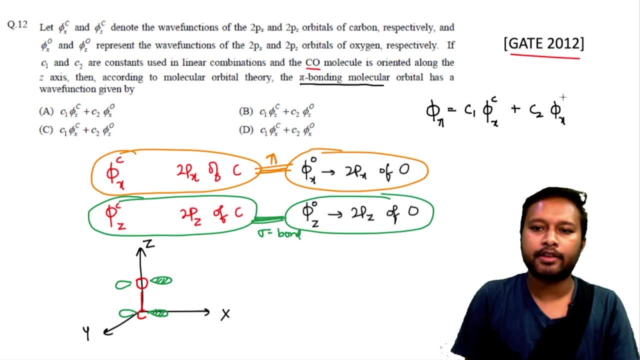 and plus c2, phi xz, sorry xo. So x orbital of your oxygen, So x orbital of carbon, x orbital of oxygen. both are going to linearly combine to form a pi bonding orbital. So that is how your option number d is correct. You just have to look upon the orientation. 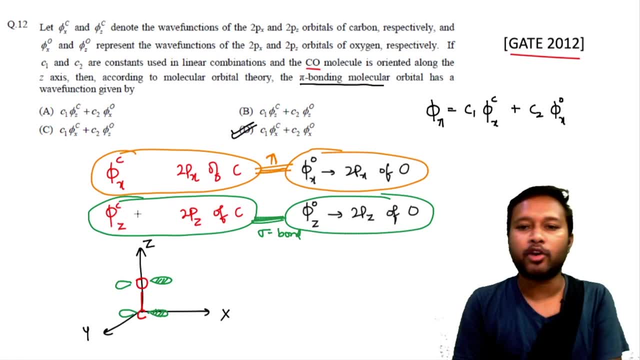 of the atom and you just have to see that which orbital will be involved in bonding, and which orbital will be involved in sigma bonding, which will be involved in pi bonding. If, let us say, the quotient, if the same quotient was for your sigma bonding, that which orbitals 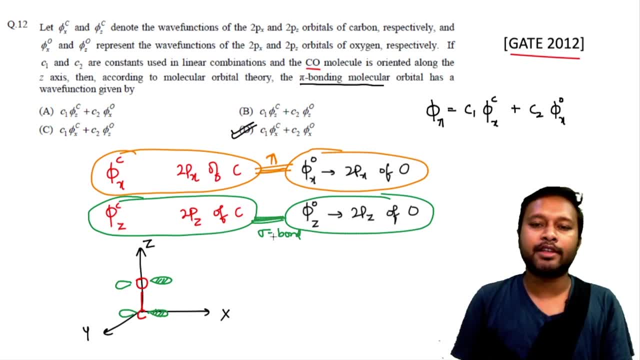 are going to be or what is going to be the wave function of the sigma bonding molecular orbital. So tell me in the comment section that which option will be the answer, a, b, c or d, which would be the answer for sigma bonding? I want answer from you guys. So 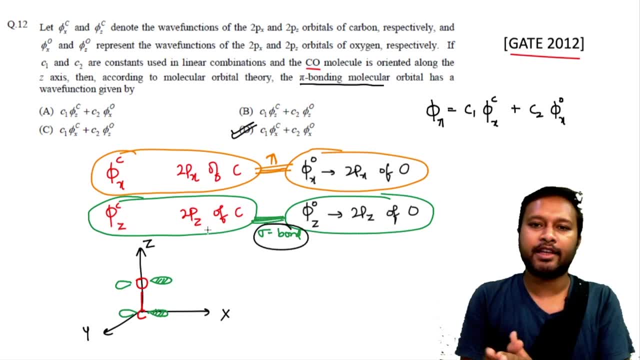 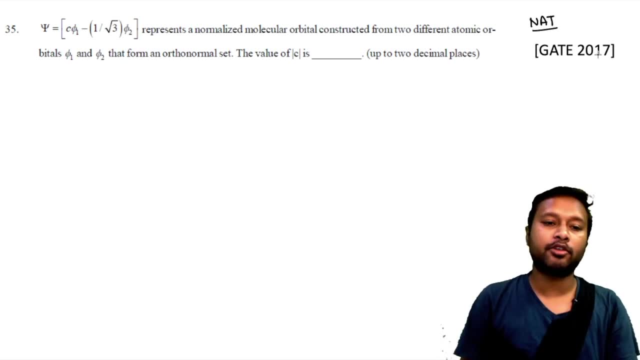 So tell me the answer for that in the comment section below. All right, let us take the next question then. All right, let us do this numerical answer type question. This is a NAT answer type question. Asdinger 2017, based upon similar concept. It says that phi is a. 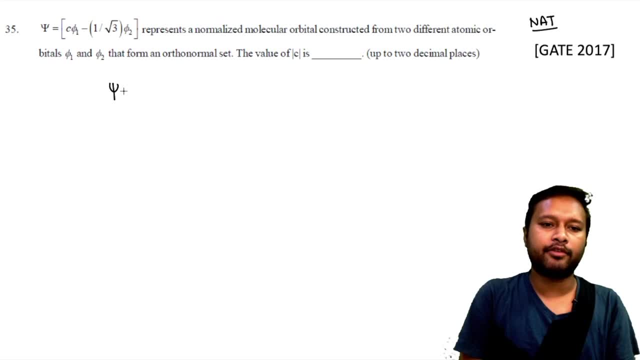 wave function, phi is equals to c phi 1.. I will write down here: phi is equals to c- sorry. psi is equals to c phi 1 minus 1 upon under root 2, sorry, under root 3, and then you have phi 2.. 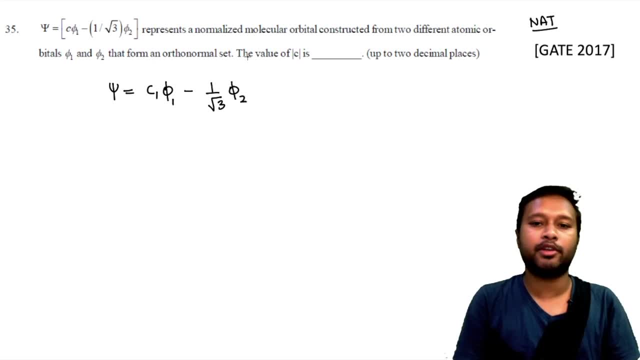 This is the wave function given Represent a normalized molecular orbital constructed from two different atomic orbitals. Orbitals are your phi 1 and phi 2.. These are two atomic orbitals. They form a orthonormal set. So what does that mean? What is an orthonormal set? So an orthonormal. 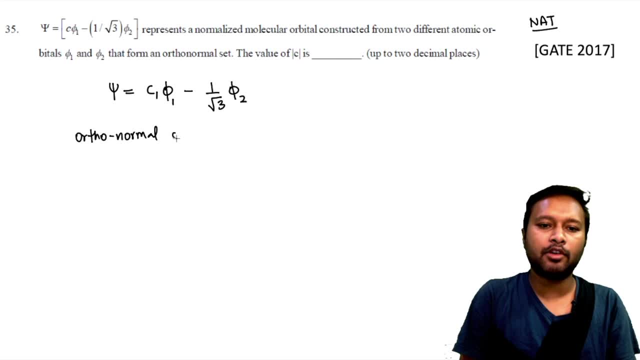 set means orthonormal set. it means that if I multiply this, like if I multiply these two wave, function phi 1 with itself, that means if I do phi 1 square, this is going to give me 1.. And similarly, 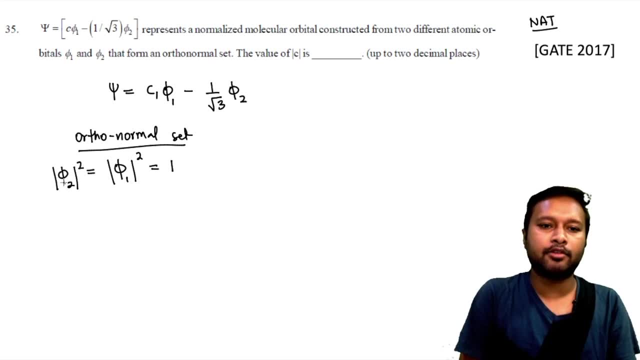 if I do this phi 2 square, this is also going to give me 1.. But if I multiply this phi 1 with phi 2, in that particular case I will get 0.. So this is normalization, this is orthogonality. 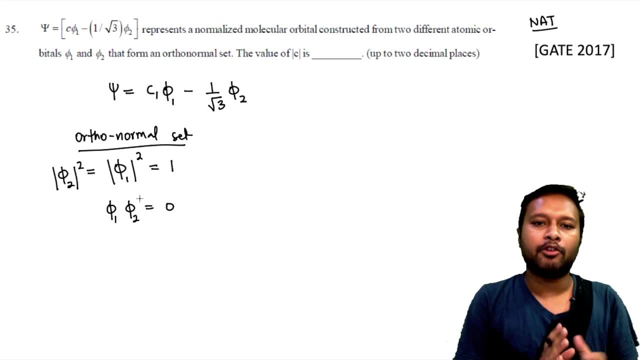 Both of them combined is called as orthonormal set. Now one thing which you should understand: that for the orthonormal set this is called as orthonormal set, So this is called as orthonormal set. For orthonormal set. they will not overlap. The overlap integral is 0 for that. So for 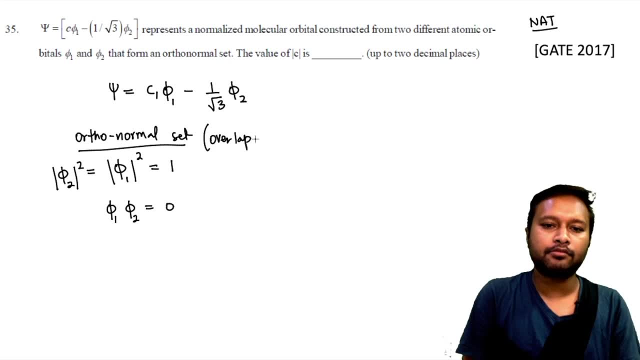 orthonormal set overlap integral is 0 because they cannot overlap. Whenever they will overlap, they will overlap destructively. So there is no overlap integral. The value of s becomes 0 in that case for all orthonormal sets. Now same concept you have to apply. They are asking you about the 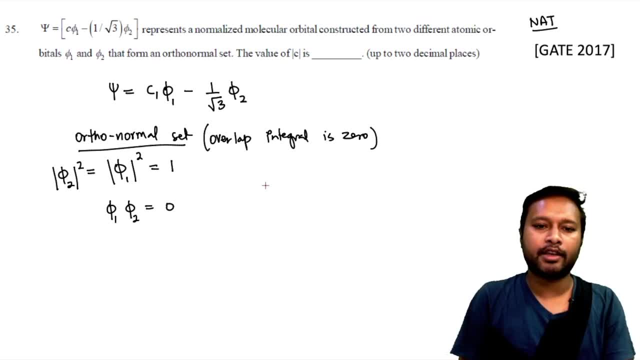 value of c. So for any wave function you know, like if I call it as c1 and if I call it as c2.. So in that case your c1 square plus c2 square plus 2, c1, c2, s should be equal to 1.. And since this is forming orthonormal set, so the value of s will. 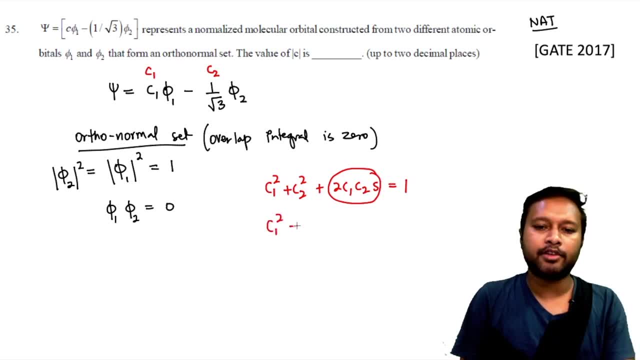 become 0. So this particular part will vanish out. You will have c1 square plus c2. square is equals to 1.. Just put the value of this: c1 has a value of c, So c square plus c2 has a value of. 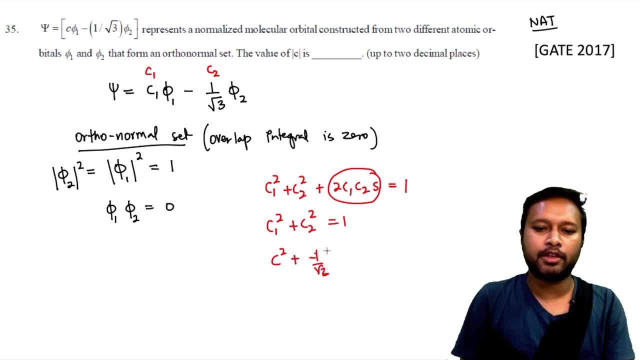 minus 1 by root 3. So minus 1 upon root 3 square, That should be 1.. Just solve it So your c square becomes 1 minus 1 square will be 1.. Root 3 square is 3.. If you solve this out, c square, 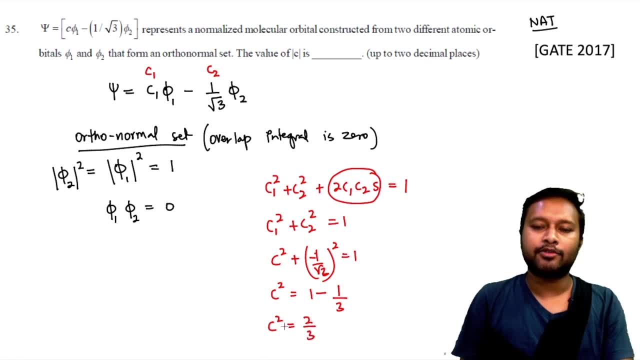 becomes 3 minus 1.. So that is 2 by 3.. So c square becomes 2 by 3, or you can say that 0.677, 0.667.. So c square becomes 0.667.. 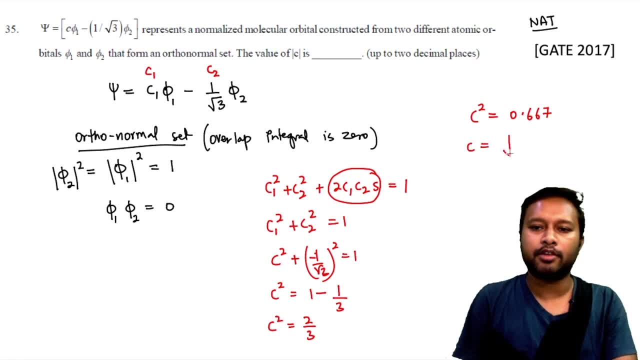 Now c will be equal to under root. It can be plus, minus both. So they are asking about the value of mod of that. So obviously you just have to take the positive value In the question. they have asked about the mod of that. So under root, 0.667.. Now do this like. use your calculator. 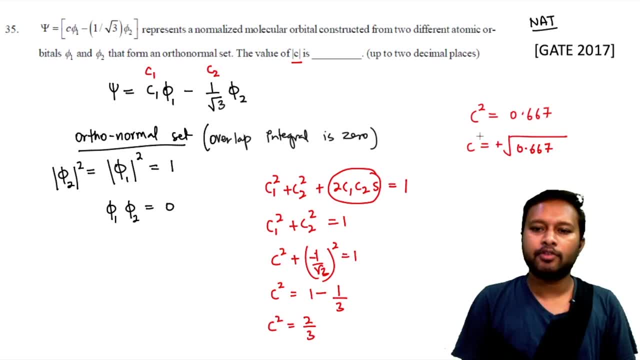 to solve it and that is what will be your correct answer for this question. So when you will solve this using your calculator, you are going to get value of 0.81.. So your correct answer becomes 0.81.. This is going to be the value of your c mod c. That is how this question has to be done. 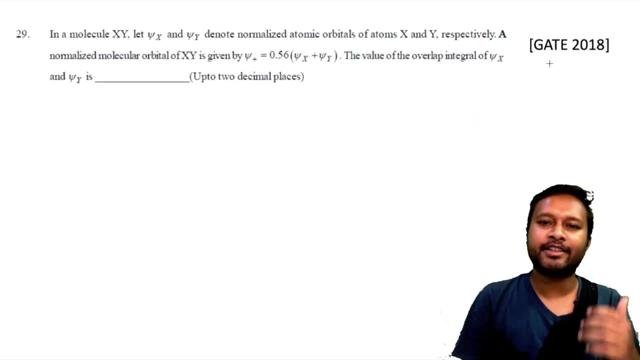 I think this is much clearer to you. Let us go for the next one, then. This is the last question for this video. It says that in the molecule xy, let us say psi x and psi y denote normalized atomic orbitals of atoms x and y respectively. 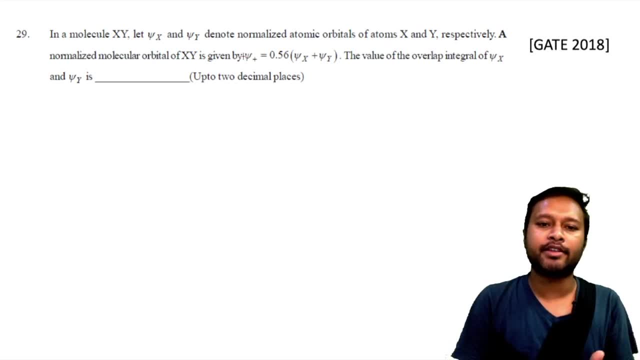 A normalized molecular orbital xy is given as psi plus and psi plus is given to you as 0.56.. In the bracket you have psi x and plus psi y. They are asking the value of overlap integral. They are asking the value of overlap integral. So let us try to solve this. What you have to 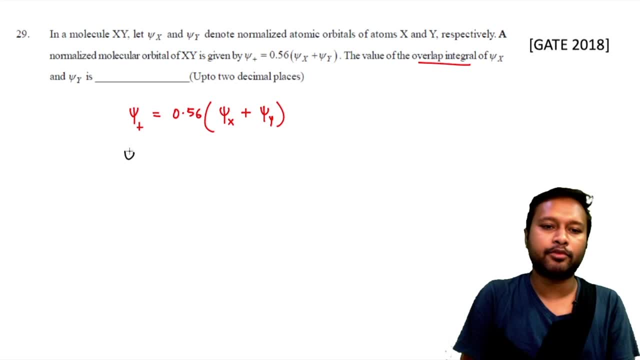 do first of all is multiply inside and make it in the standard form. So psi plus will be equal to 0.56 psi x plus 0.56 psi y. Now, if you compare it with the standard equation which we were using, 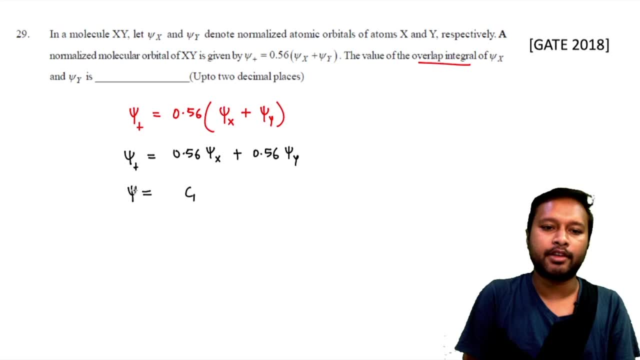 was like: psi is equal to c1.. Let us say this is phi. So phi is equal to c1 psi 1 plus c2 psi 2.. Now with that you can say simply that your value of c1 is 0.56 and the value of c2 is 0.56 again If you use the formula to. 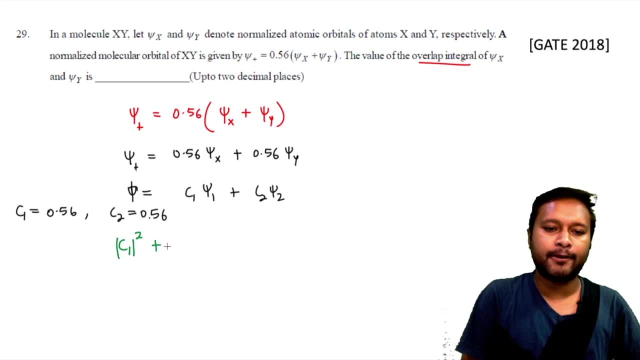 calculate the overlap integral, which is mod c1 square plus c2 square plus 2 c1, c2 s. it is equals to 1.. Let us put the value So: 0.56.. Pi square plus 0.56, pi square plus 2 times of 0.56, 0.56 and s is equals to 1.. Now you have to. 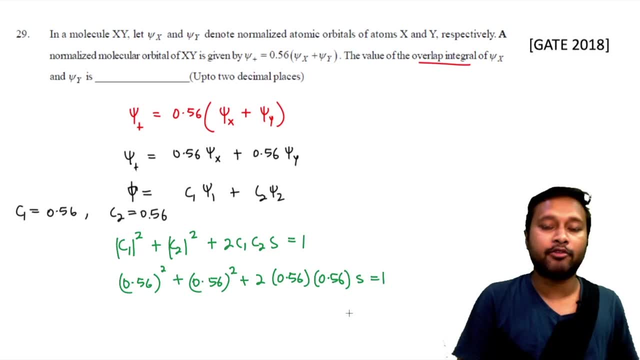 find out the value of s, So you can use your calculator to do the calculation part and you will get your answer. So I will just quickly do it and let you know. So when you will solve this whole thing you will be just getting: s is equals to 0.59.. So the overlap integral comes out 0.59.